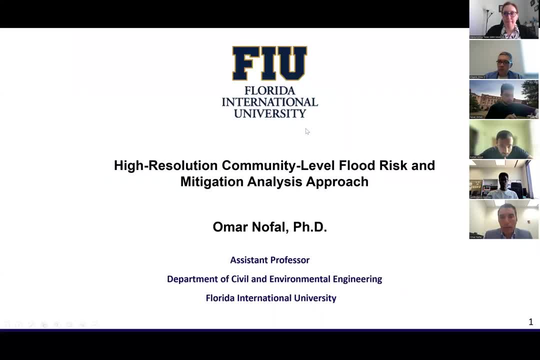 Let me get in the presenter mode, All right. So hello everyone. My name is Omar Nofal. I'm going to present a high-resolution, community-level flood risk mitigation analysis approach. So I'm an assistant professor at the Department of Civil and Environmental Engineering at Florida International University And actually 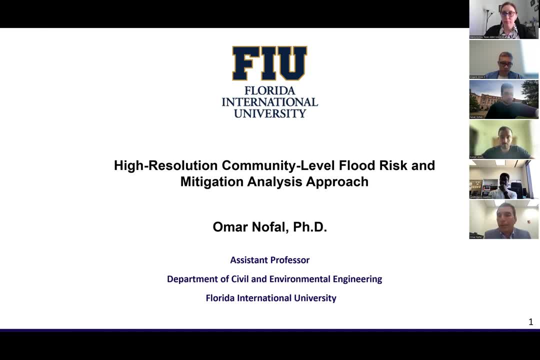 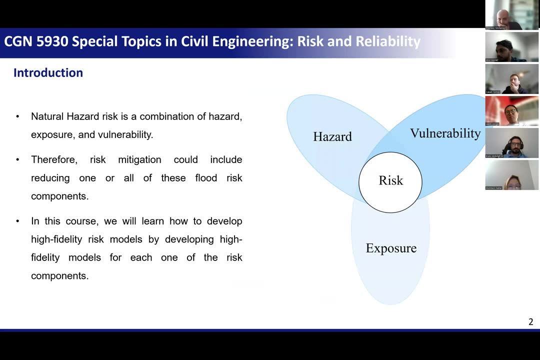 this work was part of my PhD dissertation. I have been doing this work since 2017 to 2020.. So it took me a while, but I'm going to present it so that you can have an idea about the scope of this work. Just a brief introduction about the flood risk. Actually, I was giving this seminar. 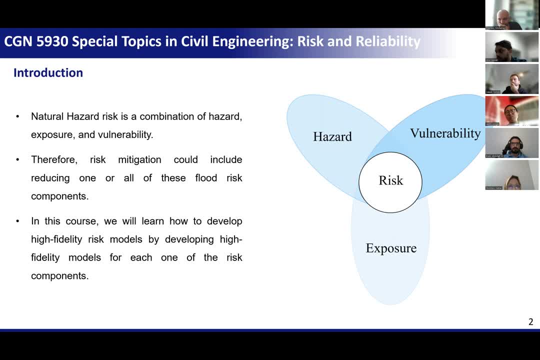 as a part of my risk and reliability class, So it's the name of my class on the top, And so for flood risk, usually when we talk about risk it's a combination between hazard exposure and vulnerability, And usually sometimes there's misconception about the. 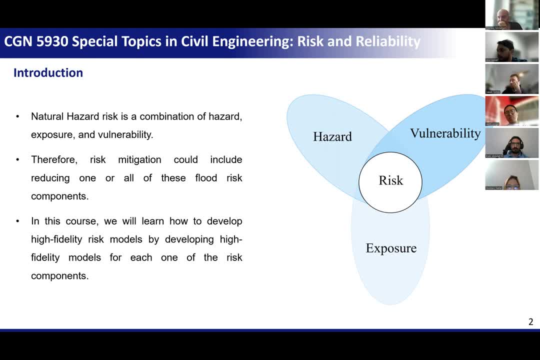 risk as just the hazard or Or the probability that you are exposed to the hazard. But here we are talking about the comprehensive definition of risk, So we are talking about your probability of getting damage from a specific hazard event to happen. So right now I'm going to present how to develop a high 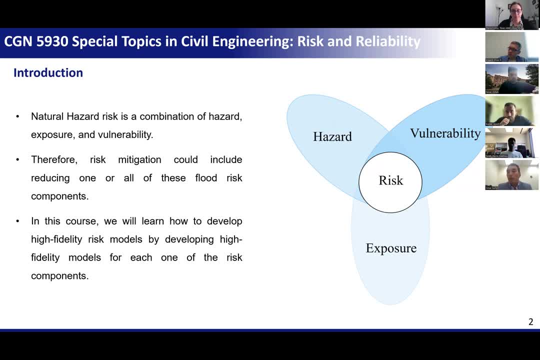 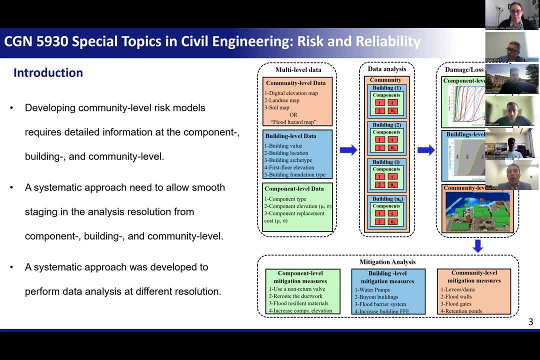 fidelity risk model with high-resolution models of the hazard, the exposure and the vulnerability of the buildings to flood hazards. So in the method that we developed we did kind of like a different resolution analysis. So we did a staging and a resolution from component level analysis to building level analysis to 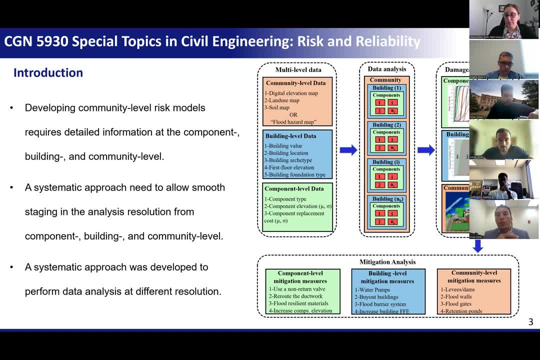 community level analysis, So the target resolution that we want to find. we need to make decisions at the community level but at the same time we don't want to lose very detailed information about the buildings and also the components. So we started to have detailed information about the 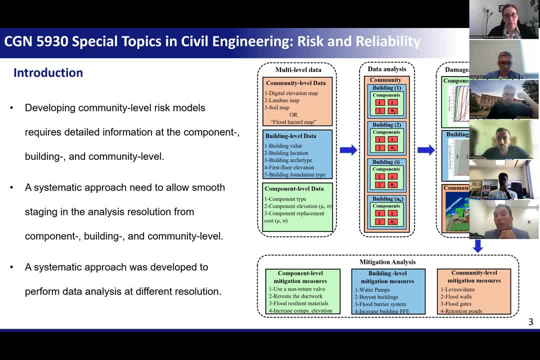 component within each building, like: what component types in each building Is there furniture, appliances, structural, non-structural components? What is the flood resistance of these components? Like what is the component elevation from the ground? What is the component replacement cost? 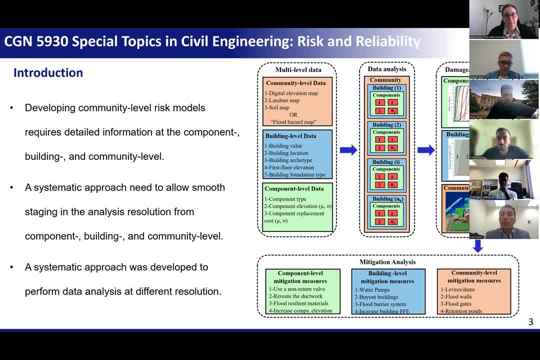 So that we can do some loss analysis. Also, each, like the different building types or the different building typologies within the community, including residential, commercial, social institutions within the community, have different component types within each building, So we needed detailed. 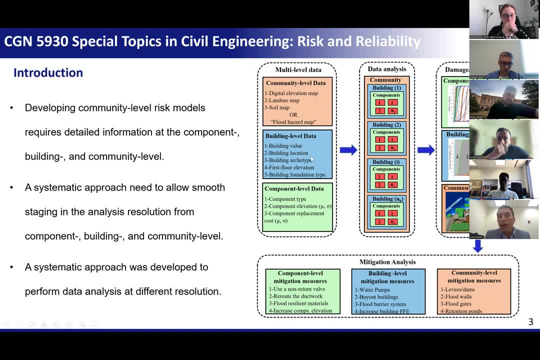 information about the buildings within the community, like the building value, the building type, the building occupancy, the building versus floor elevation, foundation type, construction material. all this information we needed about the building so that we can do building level analysis. Also, we needed information about the community, such as the: 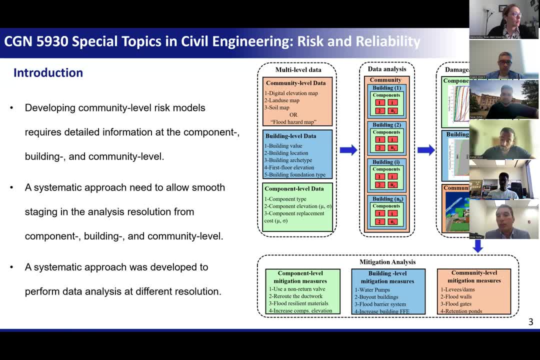 digital elevation map of the community, the land use, the soil and lots of information about the community so that we can build a community model. So that's like say that we need different types of data at different resolutions, including component building and community level. 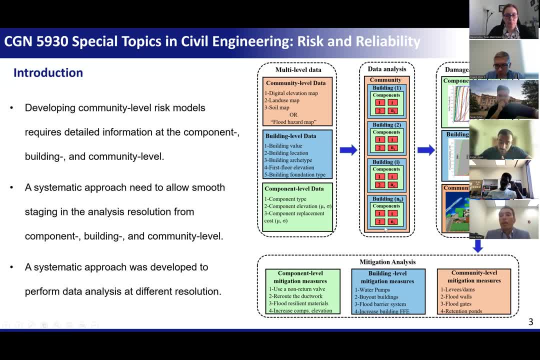 if we need to build a community level model. So- and this is how the staging and the resolution works- Like, you have some components within each building and you have building from one to up to the other, And then the community has all these buildings within one database. So this allows us. 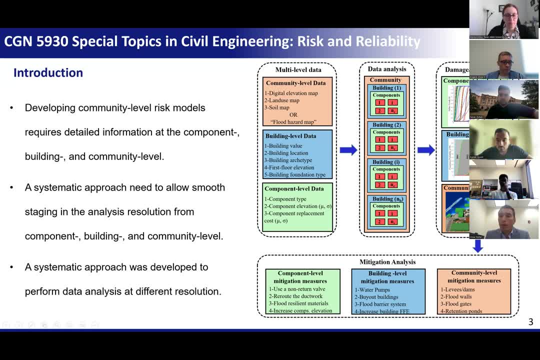 this kind of resolution allows us to have vulnerability models at the component level, So we were able to identify what is the probability of failure of a specific component within a building if they got hit with a specific flood intensity, for example, one meter. And knowing the failure probabilities of the components, we were able to identify the exceedance. 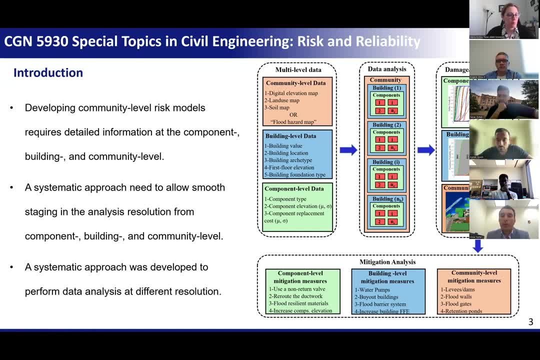 of a set of prescribed damage states for a specific building. For example, if we have a residential building, we were able to know what is the probability of this building having a slight damage state or a moderate or extensive damage, or even a complete damage. 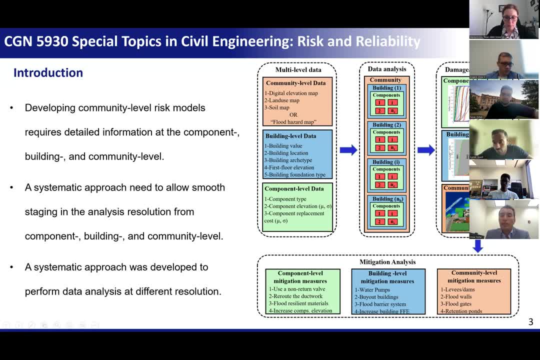 And then we developed an approach to extend the developed method from the building method to identify the vulnerability of the community, which we are going to show later in this seminar, Doing such a staging in the resolution from the component level to the building and the community level. 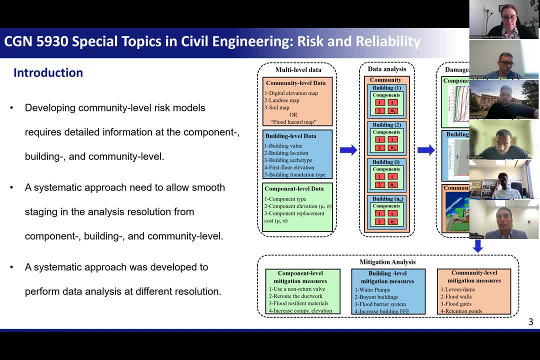 allows us to do some investigation of mitigation measures at these different resolutions. Like, for example, households during flooding. they do some mitigation measures but nobody has investigated what is the impact of these mitigation measures on the total loss, Like, for example, if a household knows that there is a flood is coming. 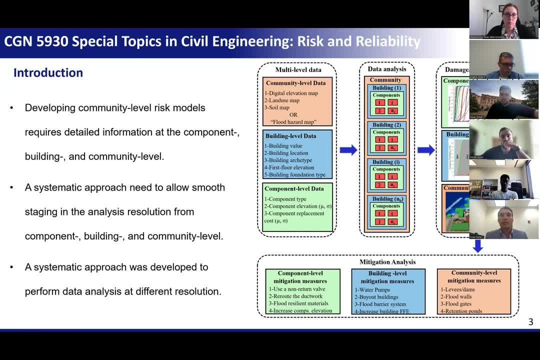 in like a couple hours or four hours and he starts to put some sandbags having a bomb or something elevating the water-sensitive components like the TVs, the electronics, the gadgets and all the stuff. if it's got flooded it's going to be damaged. 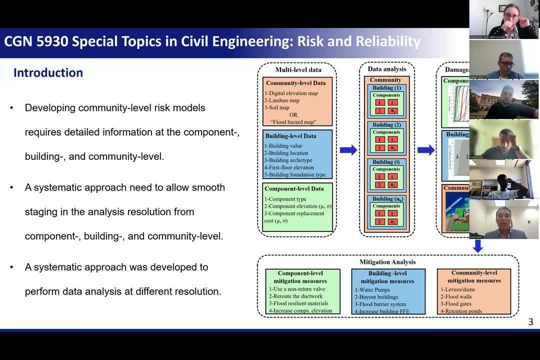 So all these can reduce the flood losses. So to capture these, we need a component-level method that can capture how the mitigation measure at the component level is going to affect the total losses at the building level and also the community level. Same approach like, in the same way we did also. 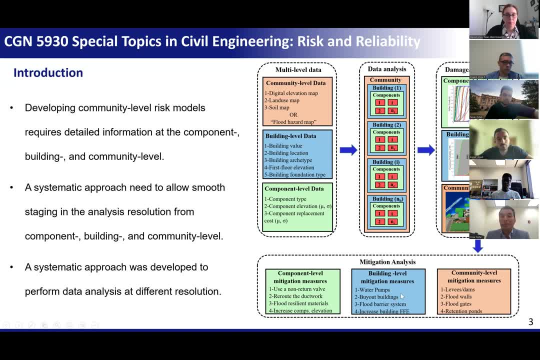 we're able to investigate building-level mitigation measures, like, for example, if you have a flood barrier system around your building, how this is going to impact the building losses. if you were able like, if you did, mitigation measures such as increasing the various floor elevation. 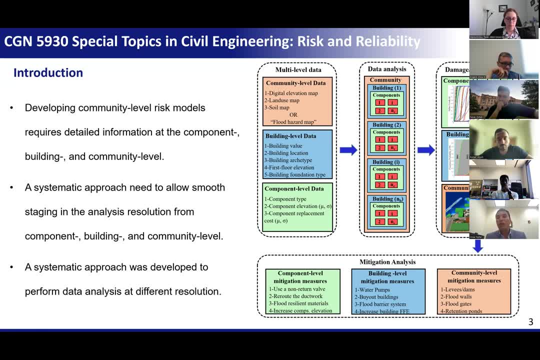 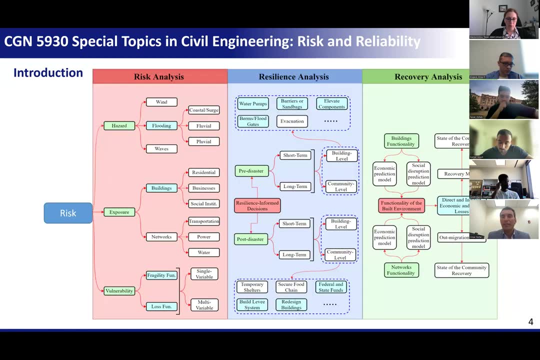 of the building having water bums, and also community-level mitigation measures including levee system, flood walls, a floodgate, retention systems. all these has been included in this study, So having such approach allows us to expand the scale of our analysis. 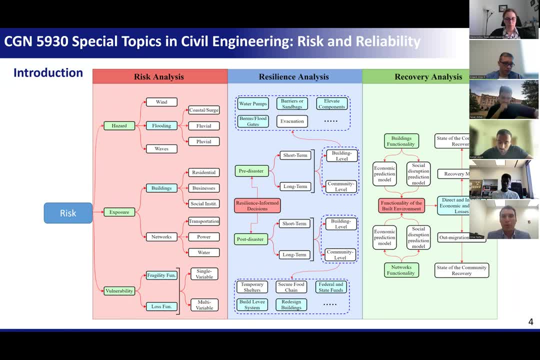 We were able to do detailed risk analysis at the component building and community level and also do community resilience analysis and also can pass the way like can pave the way to do recovery analysis for the entire community. So for the risk analysis when we talk about, like, hurricanes. 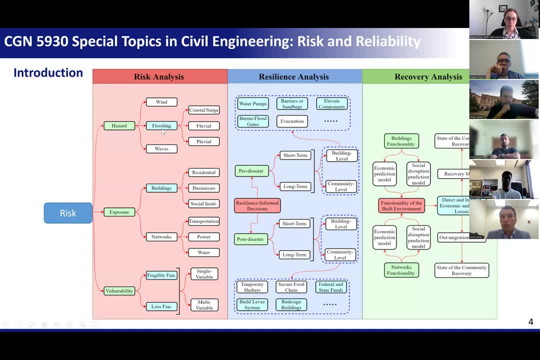 we are talking about. we have multiple hazards and one of them, which is the focus of this lecture, is the flooding. If we're talking about exposure, we can study the exposure of buildings or networks, but we are focusing right now on buildings. 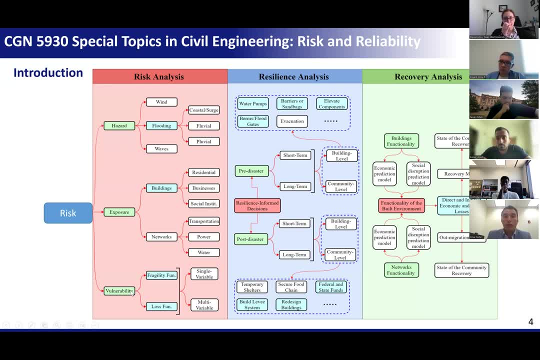 including residential, commercial and social institutions, And there is different way to quantify the vulnerability of these buildings, either using fragility functions or using loss functions For resilience analysis. with the approach that we have used, we can investigate different resilience and forming decisions either pre-disaster or post-disaster. 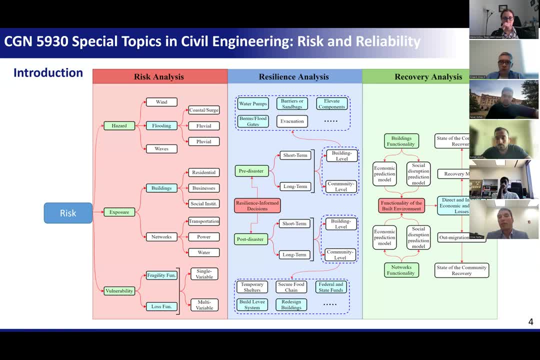 at the short-term or long-term, even at the building level or at the community level For recovery analysis. you can, with the approach that we develop, we can track the functionality of the built environment, what is in terms of social functionality, and also the physical functionality. 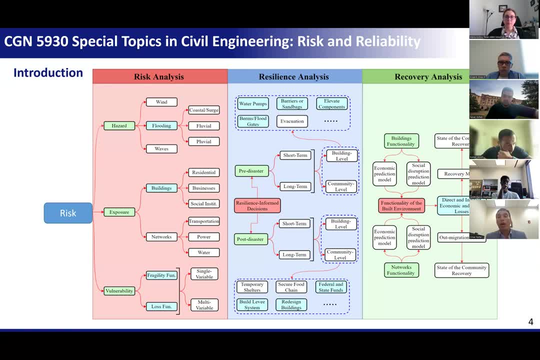 of the entire community and link multidisciplinary models in the physical models that we develop, Like if we know the damage, we can know how much economic disruption that we are going to have and link this damage with some social models to identify. 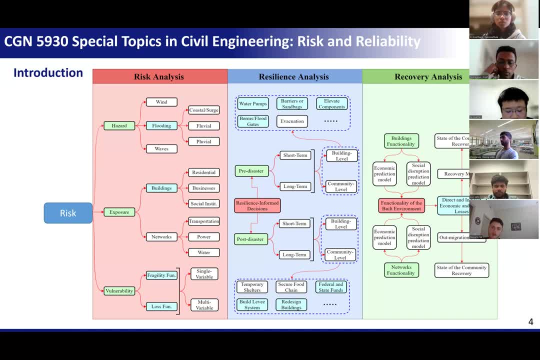 the population dislocation and many resilience metrics we can measure using such models. We applied this to different hazard types. This includes the flood hazards and also multi-hazard hurricanes, Like if the hazard is combined with wind. like what if we have wind and also storm surge and waves? 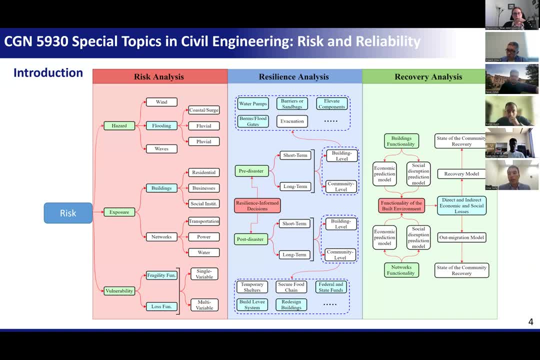 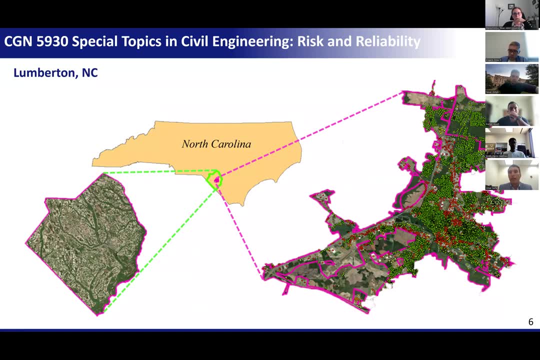 how all these combinations are going to affect buildings. But right now we are focusing on flood risk analysis. So an example for the flood risk analysis we use is we used Lumberton, North Carolina. So Lumberton is a small city within Robeson County. 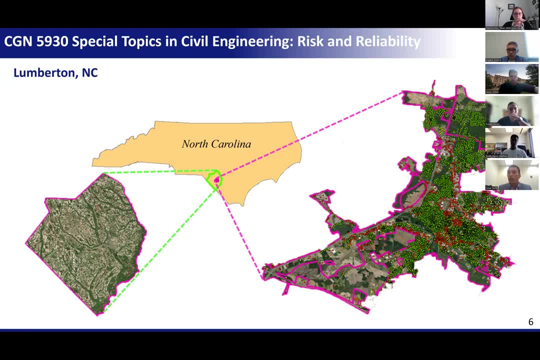 in North Carolina We have detailed information about the buildings within Lumberton, So this includes the. actually, the entire state of North Carolina have very detailed- and also one of the most detailed- information about the buildings. They give you, for example, 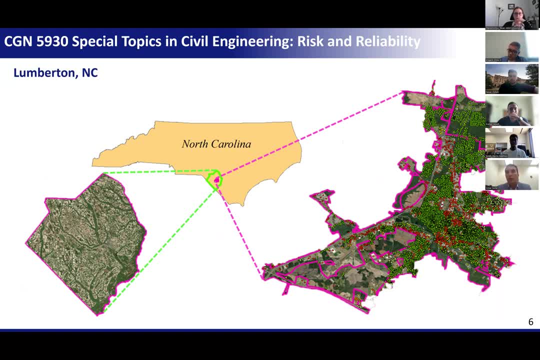 the roof type of each building and how many shingles on this building and how many nails in each in each building. So it gives you very detailed information, including various floor elevation, construction material, foundation type, which is very important if you want to have. 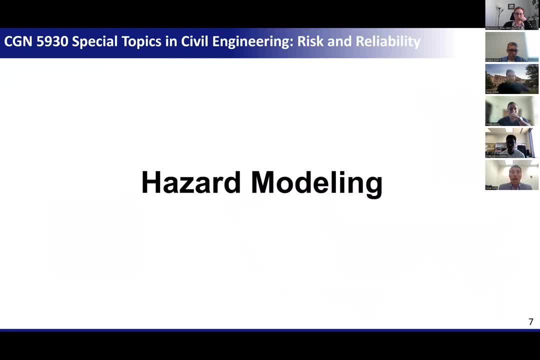 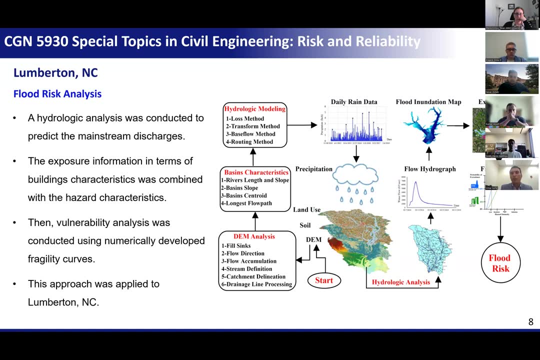 a high resolution model at the building level For the hazard model that we study for Lumberton. so for hazard modeling we developed a high resolution flood risk model that combined hydrologic modeling with hydrodynamic modeling. So hydrologic modeling was done like. 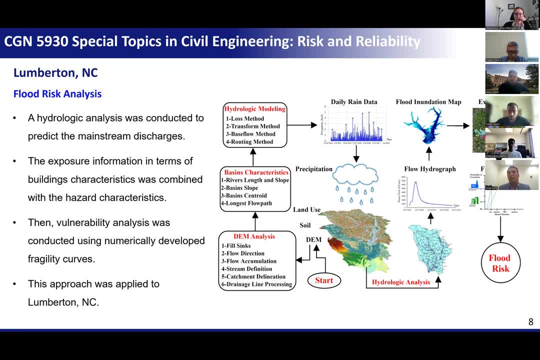 using like a bunch of methods, which is a typical hydrologic modeling. They use detailed information about the rainfall, the land use, the soil, the digital elevation map so that we can identify the water flow in each major stream in the study area. 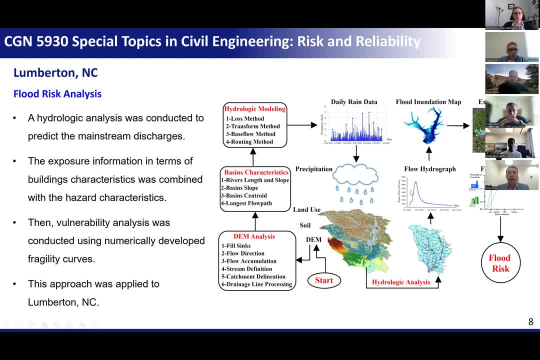 Once we identify this water flow, it's usually in terms of a hydrograph. This hydrograph is like: how much is the water flow in each stream over time across the course of the the whole flooding events? So, as in any flooding event, 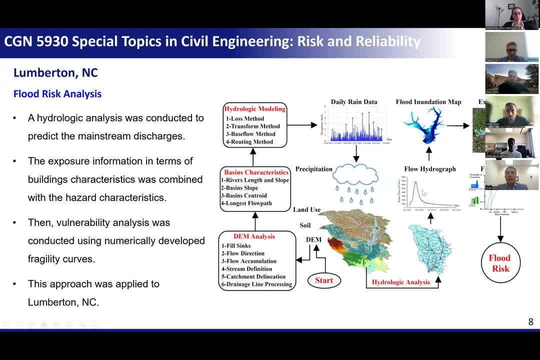 you always have the water flow start slow and then it jump and then it goes slowly once the event is done. So the water flow peaks and then it goes back to normal. But the idea is not only to get water flow. we need to know what is the flood inundation. 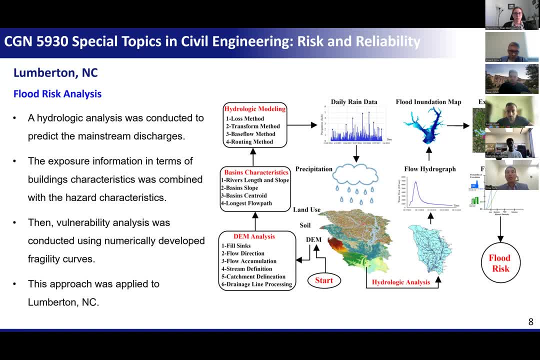 across my study area. So we need to do hydrodynamic analysis to convert this water flow into a flood hazard map. So a hydrodynamic model was conducted And then, once we have the flood hazard map, we overlay it, which is a detailed community model. 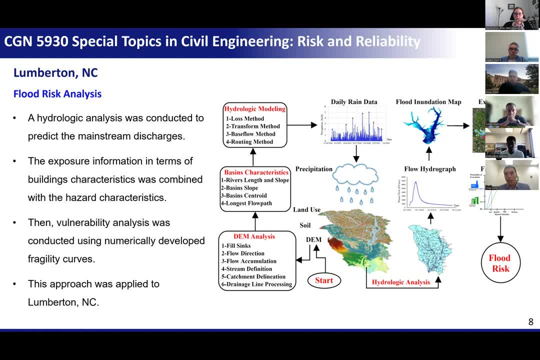 to identify what buildings that are exposed to flooding And what is the level of exposure, Like what is the flood hazard intensity at each building. Once we know the flood hazard intensity of each building, we use what is called the fragility curves to knows what is the level of damage. 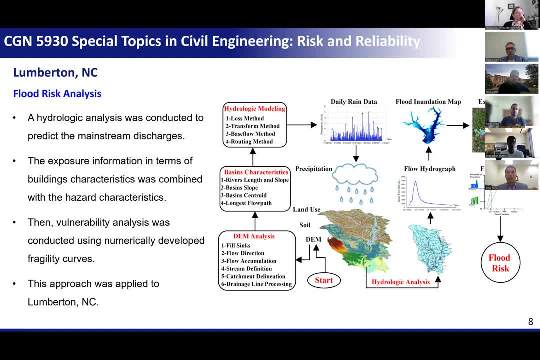 for each one of these building, corresponding to each level of exposure. Like, if you have a flood, that's two meter, you will have this amount of damage. If you have one meter, you will have this amount of damage. So we applied this approach. 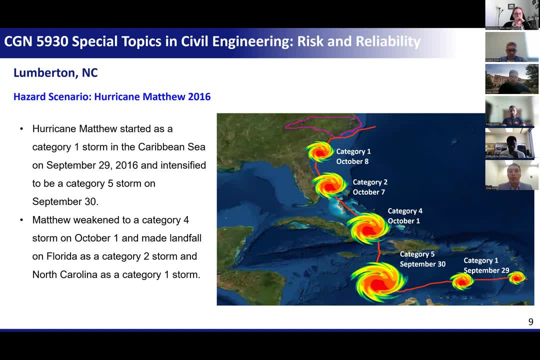 for the Lombardy, North Carolina, as I said, and we used Hurricane Matthew in 2016 as a hazard scenario. So Hurricane Matthew started as a category one storm in the Caribbean and then intensified to be cat four, but at the landfall it was a category one storm. 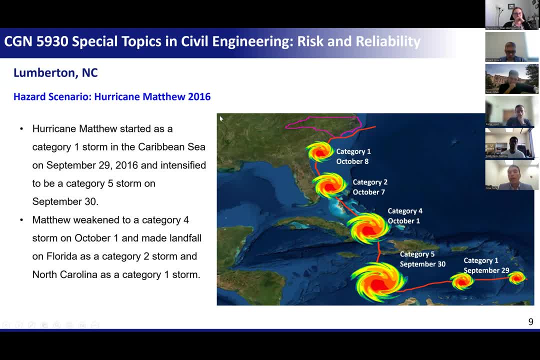 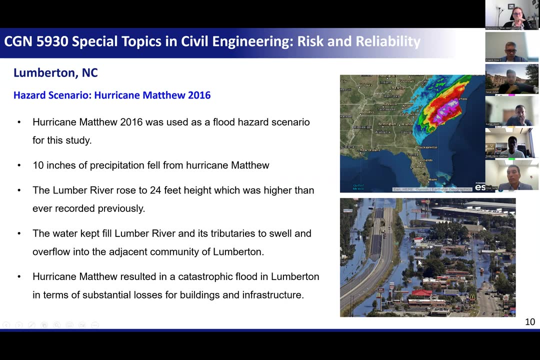 It made landfall on October 8th in 2016.. And it was actually. there was a coastal flooding, but also there was river rain. flooding comes in from the, the heavy rainfall, So this is one of the locations in the downtown Lumberton City. 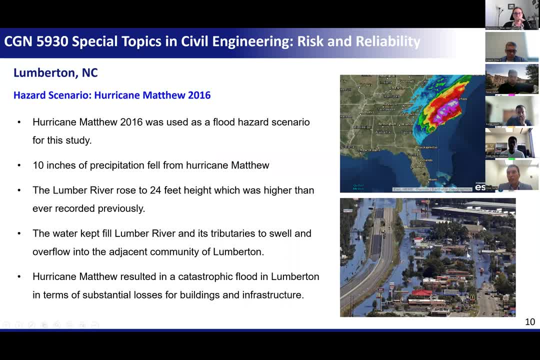 So it's. how's the flooding look like across the city? Many businesses, residential building got flooded And this map is from NOAA that shows how much is the rainfall intensity across North Carolina or across the United States. actually, The maximum was here, whereas Lumberton at. 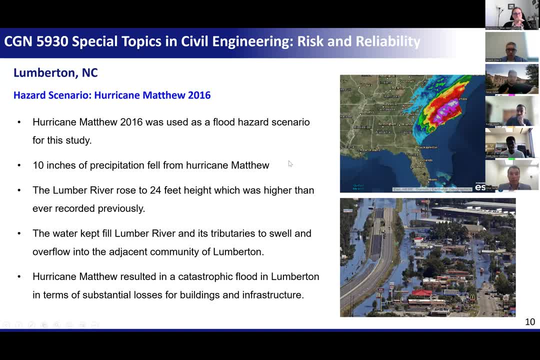 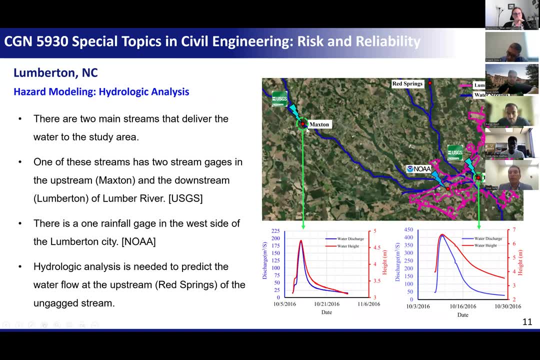 which is more than 10 inches of flooding. So for the hydrologic analysis for this study area, so we were able to get the flow hydrograph at the locations, or what we call is the upstream. So this shows how much is the flow and also the gauge height here at this locations. 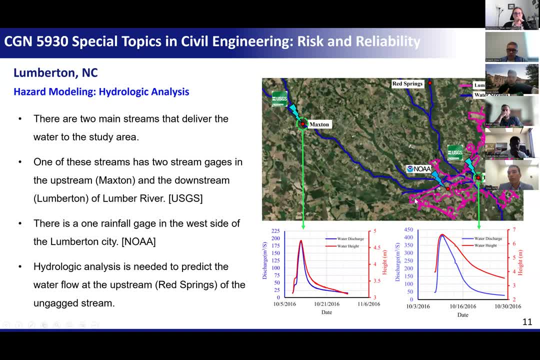 This is upstream of Lumber River and this is downstream of Lumber River. So here it shows how is the water flow: jump it from 25 meter cube per second to almost 200. So it's like eight X, like the normal flow. 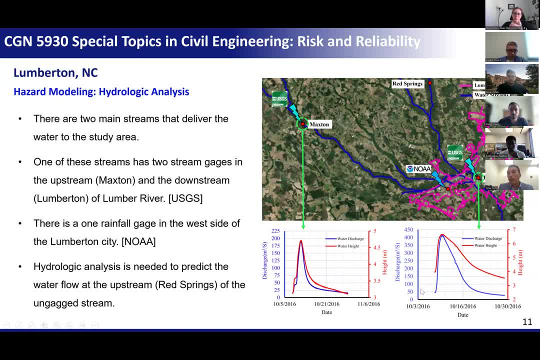 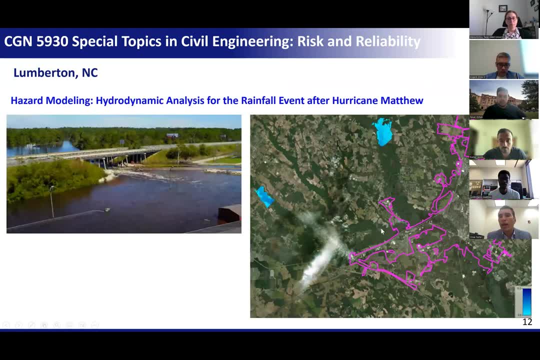 And also the same thing downstream from 50 meter cube per second to more than 400 meter cube per second of water, And we use this hydrographs as a boundary condition for hydrodynamic analysis. So basically, we put this hydrographs here as a boundary condition and run a hydrodynamic analysis. 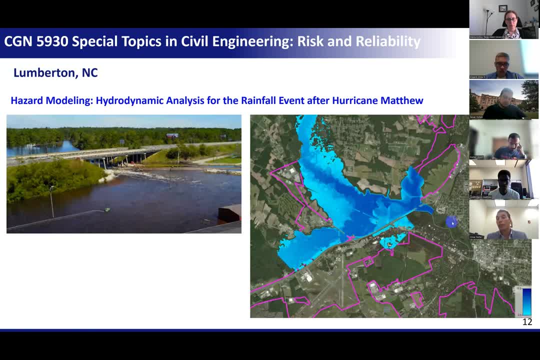 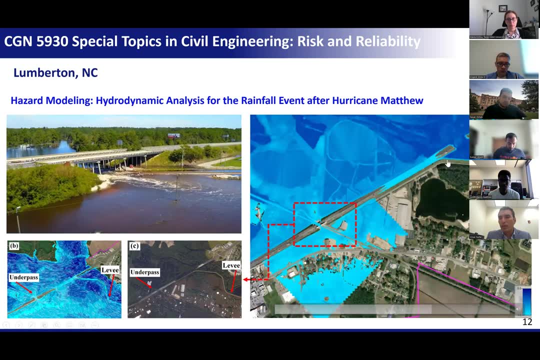 that solved the San Vinan flow equation, like a shallow water equation to identify the water depths. And here it shows one of the main locations Like: if you see here, you will find that we have a levee here that retains the water. 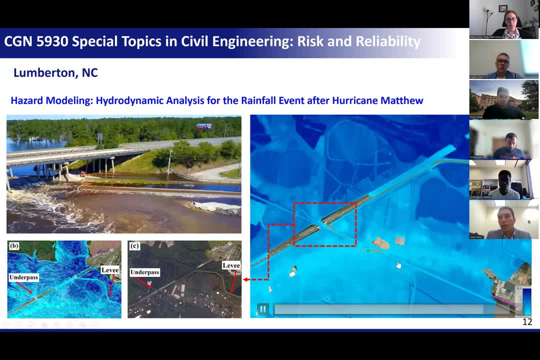 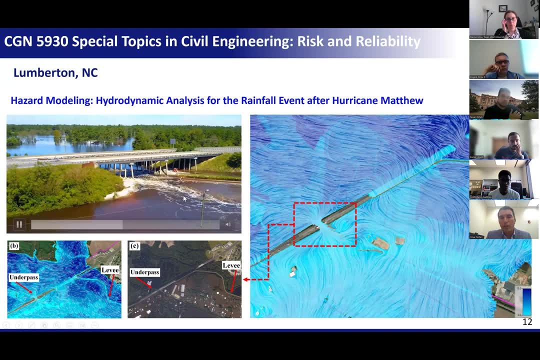 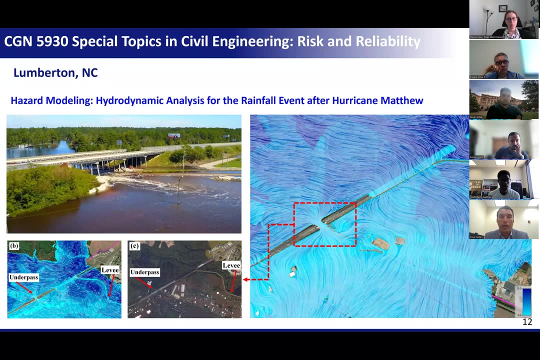 but we have a weak spot here that allows the water to go inside the city And on the left side it shows where is actually this spot at and it shows how is the water made it in the downstream. So this is one of the weak spots that allows the water in. 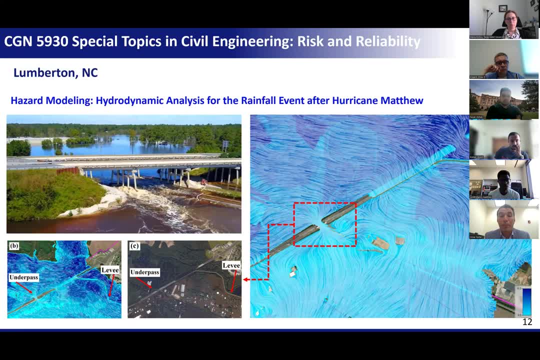 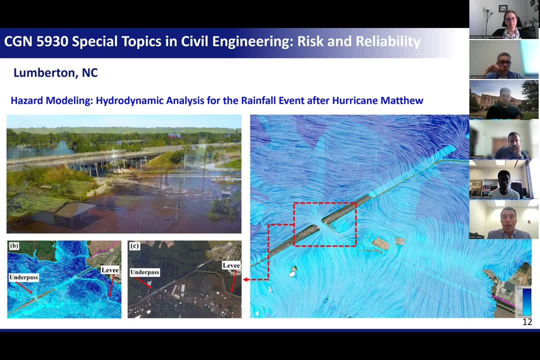 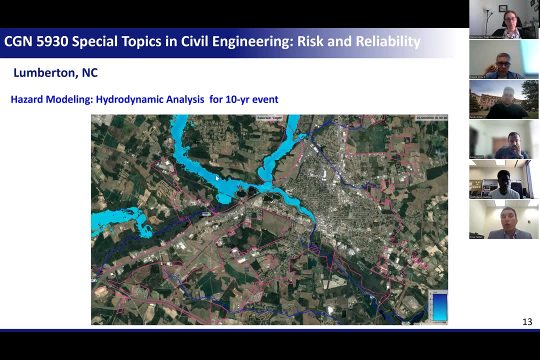 And this is one of the things that we are studying as a mitigation: What if we built a gate here? how much flood protection we can provide to the community. So after the flood hazard mapping, we mapped the flooding event after Hurricane Matthew, but also we did some return buried events. 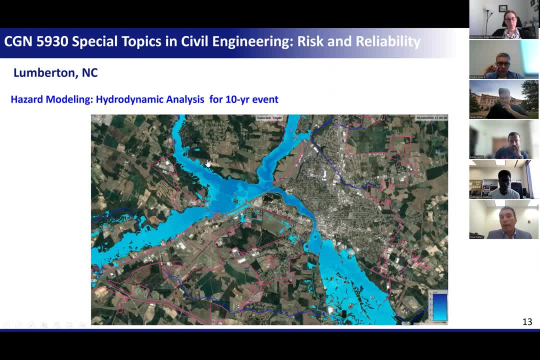 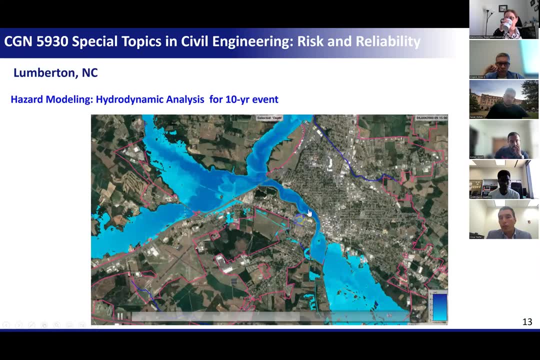 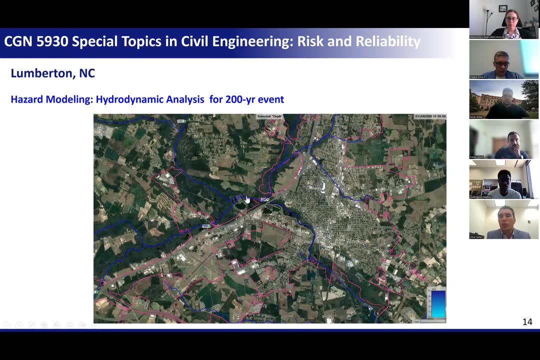 So we studied what if we have a 10 year event. So here's: it shows like there's minimum amount of flooding, just like the water flow in the river regions and didn't make lots of flooding within the study area. But if we look at the 200 year event, 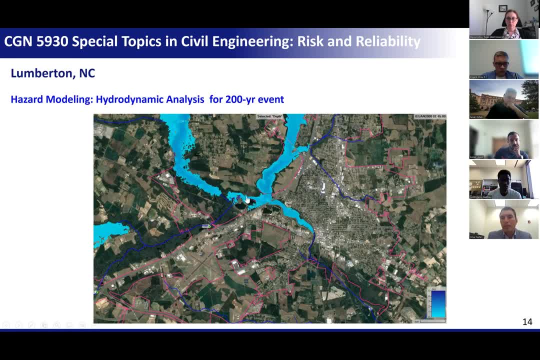 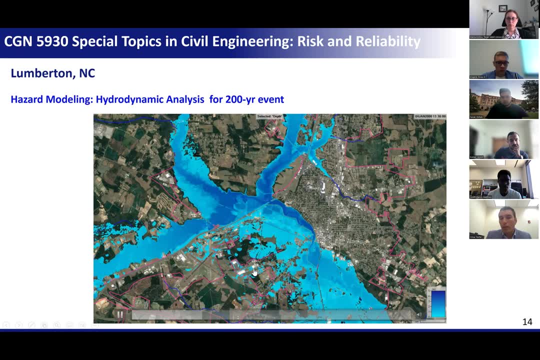 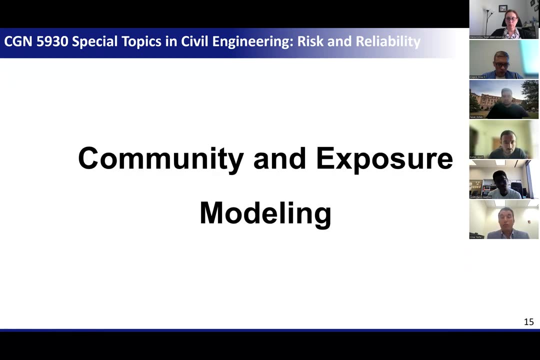 which is like almost a typical to Hurricane Matthew. So you will find that was a 200 year event. You will have much more overflow here within the south side of Lumberton community. So after modeling the hazard, the next step is to model the community. 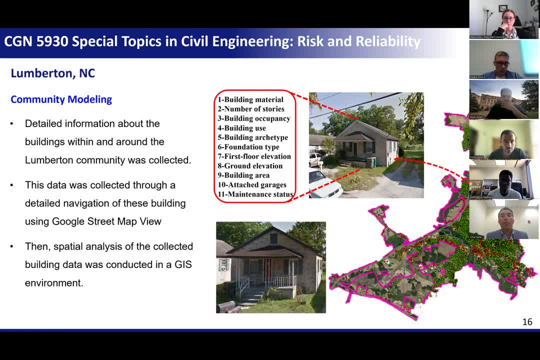 So to model the community, we need to have detailed information about the buildings, where they are: what is the building material, the number of historic occupancy, use, foundation type. We were able to have all this information. We collect some of this information. 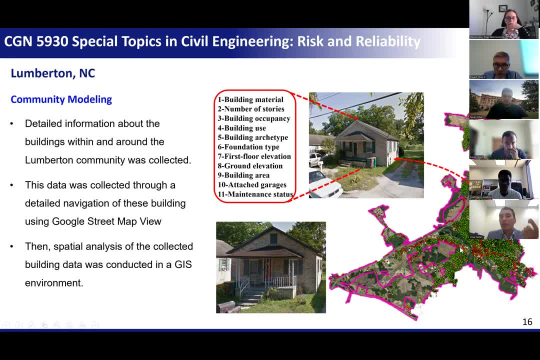 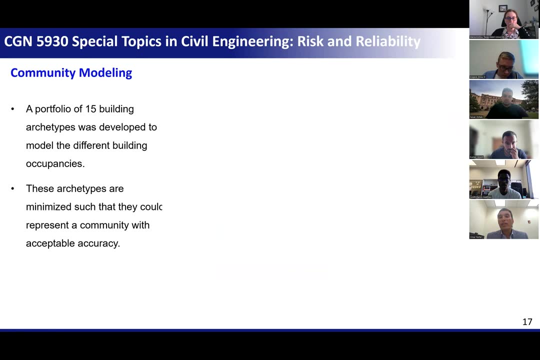 from Google street map view and also we're able to have this information as a GIS layer provided by the state of North Carolina. So, using all this information about the buildings, we were able to categorize these buildings into archetypes, So we develop a 15 building archetypes. 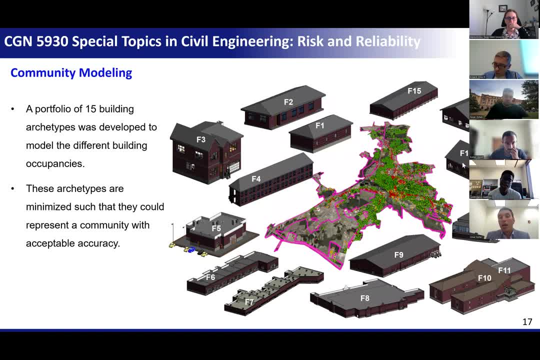 that can model the different building typologies within the community. Four of these archetypes are residential and some of these are commercial. Some of these are social institutions like hospitals, the schools, two story and one story residential buildings, the strip malls. 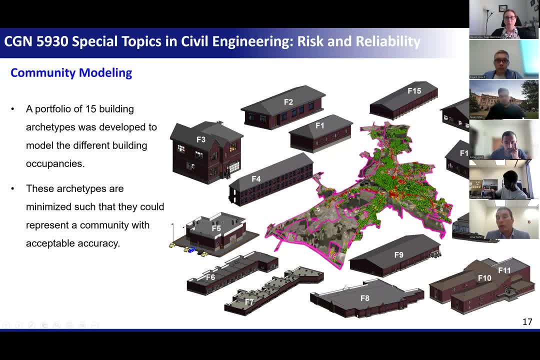 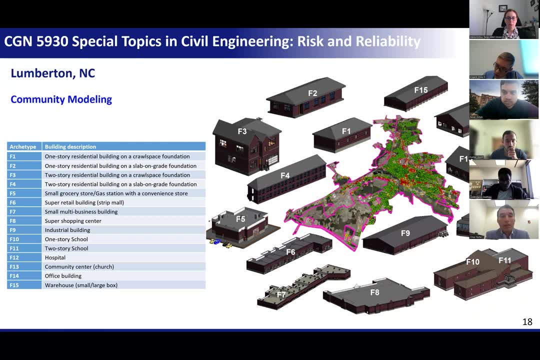 shopping centers like Target and Walmart warehouses. So we have these 15 building archetypes to represent most of these building typologies. So here's the name of these archetypes, like from F1 to F15, along with detailed description of each one of these archetypes. 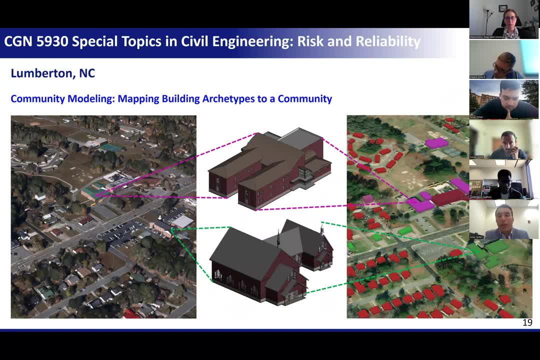 And then, after we develop these archetypes, the next step is that we need to identify, based on each building information, what is the building archetype for each real building. So we have 15 building archetype and we have the real community. We need to assign these 15 archetype. 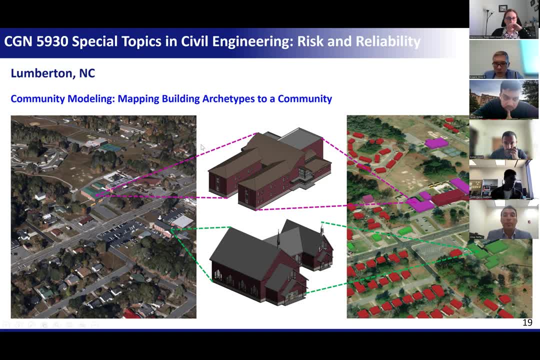 to the real community. So we like develop the mapping algorithm that use the detailed information provided for the building and assign an archetype for each building, Like. it's kind of like a, a Bython code that makes some F statements If this building is a one story. 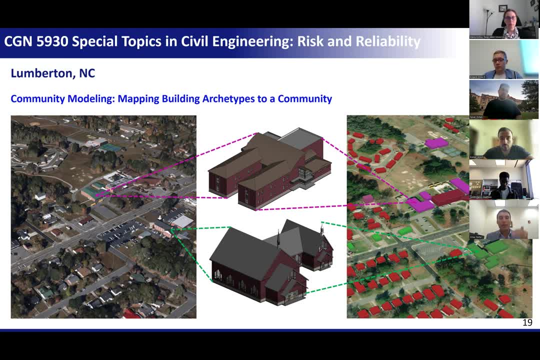 on a crawl space foundation and it has this type of information assigned archetype one. if it's two story, archetype two. so it's kind of something like this. So on the left side we have the, the real, the real community. 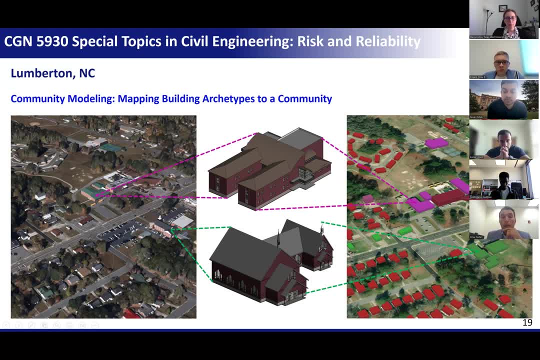 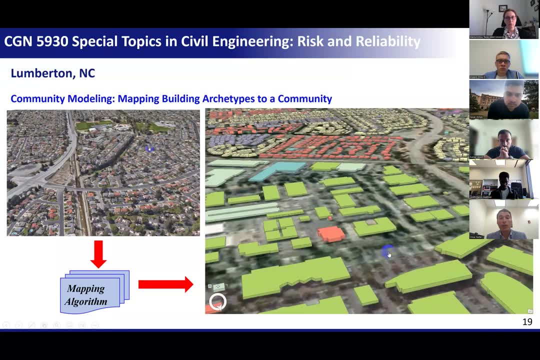 And on the right side we have the map community After that. so we applied this approach, like for many communities, like applied this for Santa Clara County, California, Long Britain, North Carolina, Waveland, Mississippi, like many states around the US. 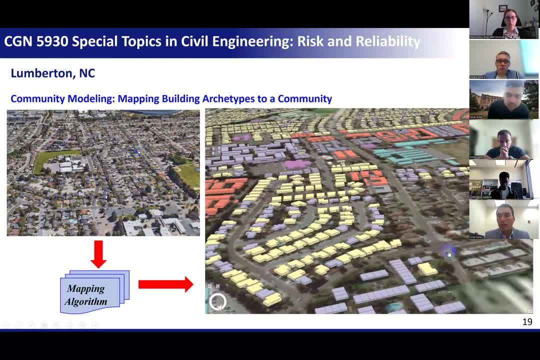 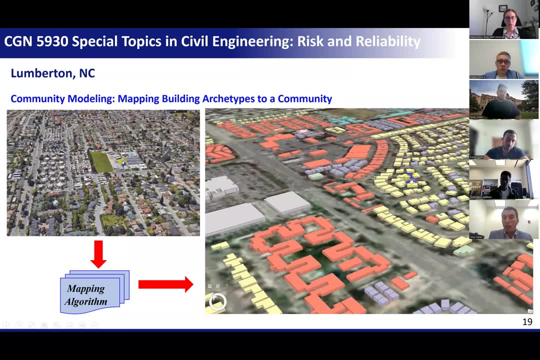 So here's it shows how's the mapping look like, How's the. so these are. all of them are buildings, color coded based on their archetype. And once we map the community, the second step is that to overlay the hazard map that we developed, 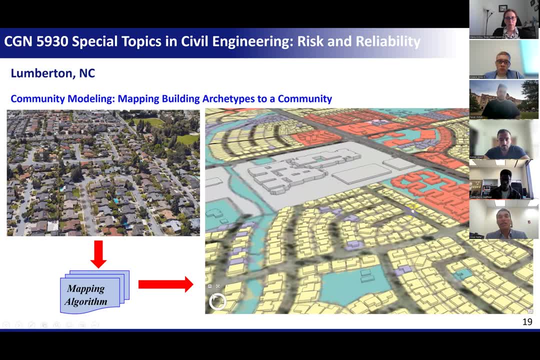 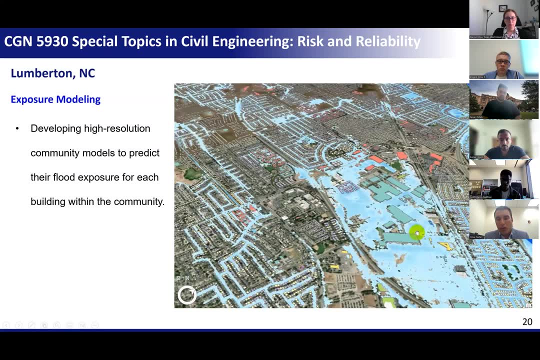 with the community that we have and identify the hazard intensity at each one of these buildings. So here's it shows in 3D the hazard map overlaid with the community model that we developed And based on this we can do some spatial analysis. 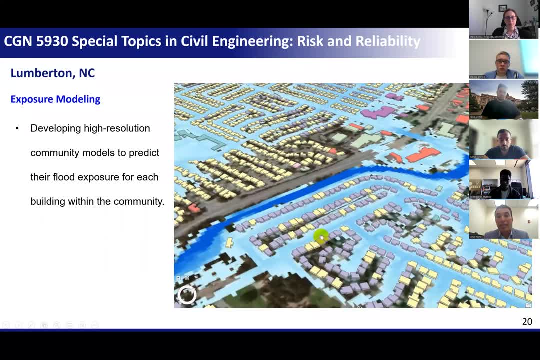 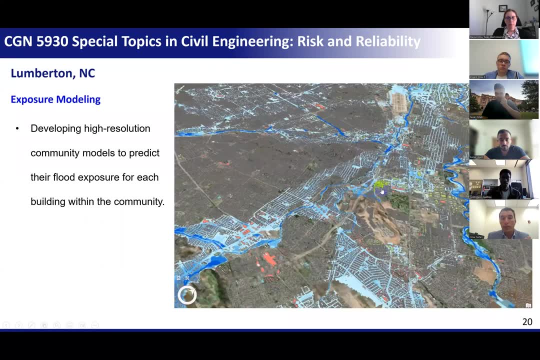 to basically identify the hazard intensity at each one of these buildings. So right now we are done with the hazard modeling, exposure modeling. So the next step is: once we know the hazard intensity, how can we know the damage for each one of these buildings? 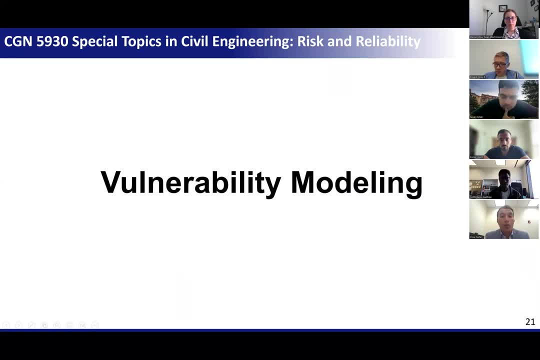 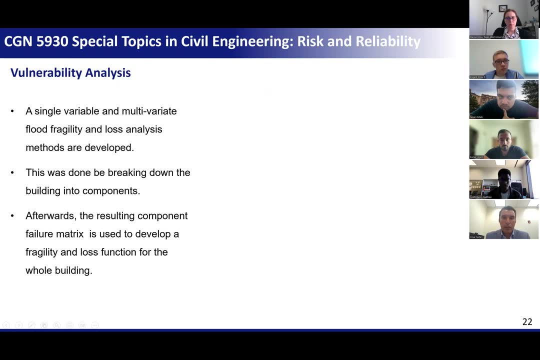 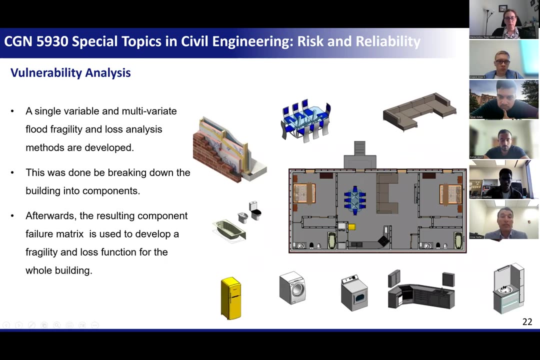 For this we developed a new approach for vulnerability, flood vulnerability modeling. So, basically, for each one of the archetype- the 15 archetype that I showed to you- we divided the building into components, identified all the components within the building and studied the flood susceptibility. 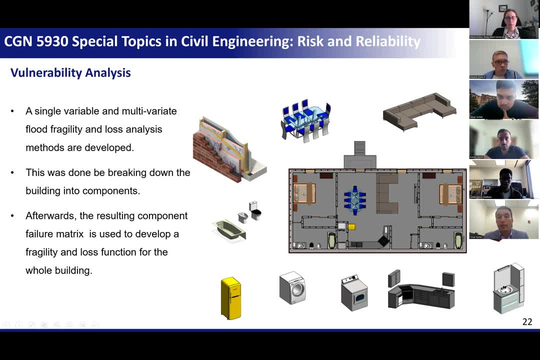 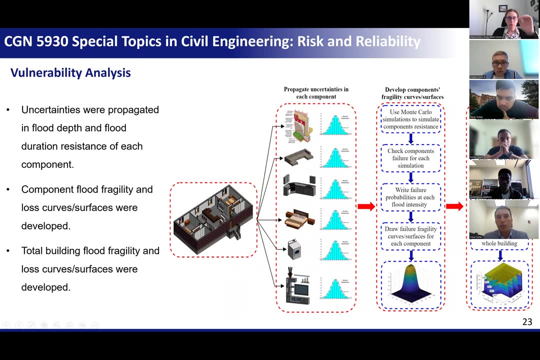 of each one of these components, including content, this furniture, other components, again, appliances, structural components like dry walls, flooring, roofing, roof sheathing, isolation. all the component was in the building and then we developed a component-based approach that can tell us what is the probability of failure of each one of these component, based on the susceptibility of each one. 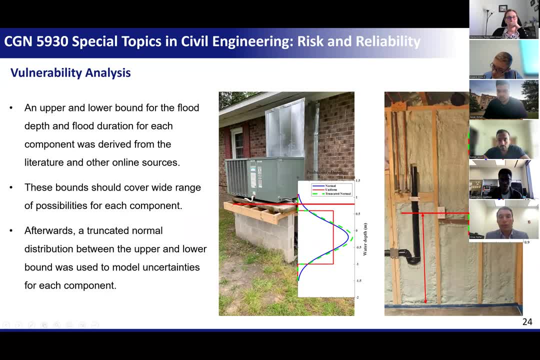 of these component water. so here's for example that shows, for example, the ac unit. so so ac unit is like is a water sensitive component. once it got touched with water it will be out of service. but the uncertainty is in the elevation of this component. so this component could be on the ground. 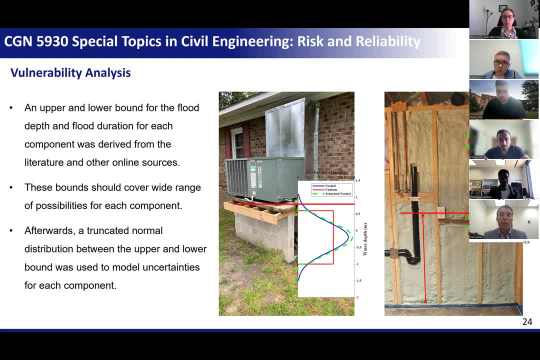 could be elevated from the ground. so this picture actually from lumperton, north carolina, i take it myself. so some of the homeowners were smart enough and they learned it from previous events and they elevated the components that they have. so, but some of some didn't. so we identified an upper and lower. 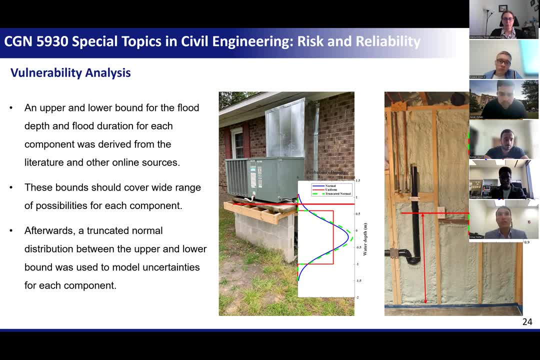 bound of the elevation of these components. the same thing can be for a tv. tv could be uh on a table or can be mounted in a wall. the table can be two feet from the ground mounted on a wall, at like four or five feet from uh the ground. so we 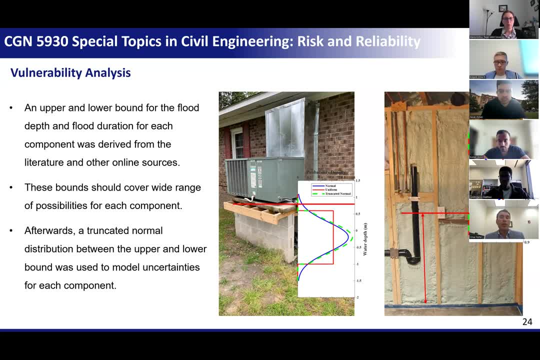 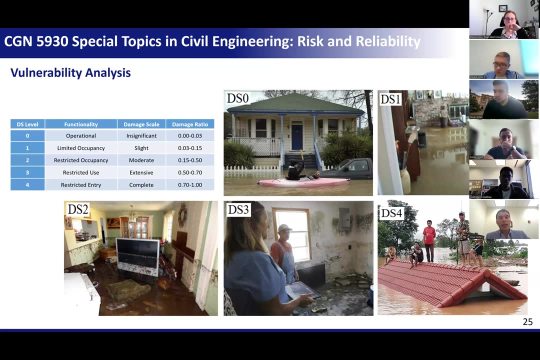 developed like we identified an upper and lower bound for the elevation of these components and we developed the truncated normal distribution and then we use monte carlo simulation to identify the failure probability of the component at different uh flood depths. so right now we have done: we identified the component vulnerability, what is the probability? 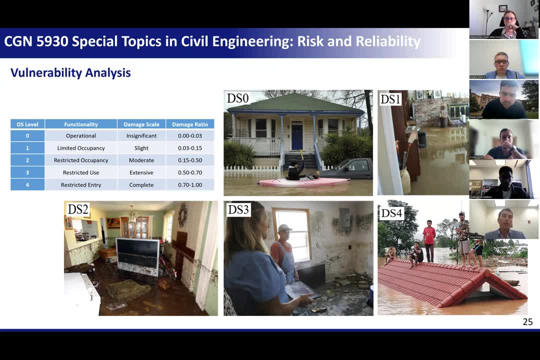 of failure for each component at different flood depths. but we need to move from component level to building level. so we developed a set of damage estates, like from damages state zero to damage state four. like damage of state zero is insignificant damage, then a slight, moderate, extensive, complete. 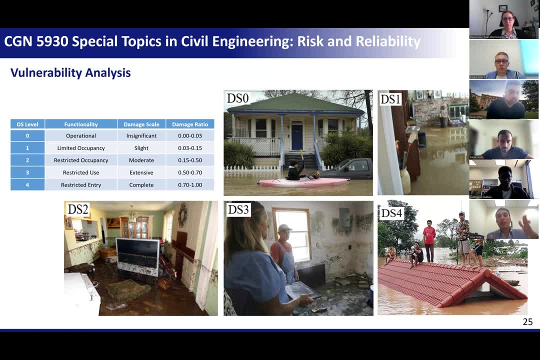 and then let's assume that our building has a hundred component. we divide these components into groups and each group is assigned by another component as a value. so that's a good case example to a damage estate. based on the failure probability of each component in a group, we can know what is. 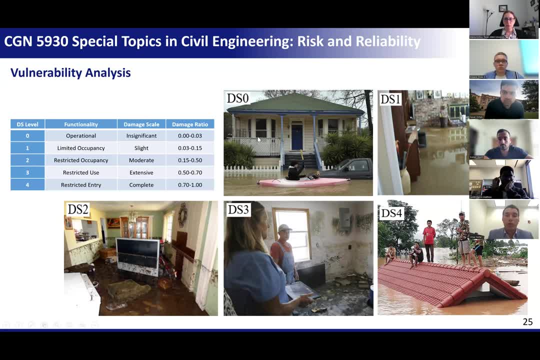 the exceedance probability of each one of these damage states. here is, for example, chose some pictures of how we consider these damages. state like: if there is no water inside your building, so you are in damage estate zero, but damage estate one is like one inch inside the building, so you 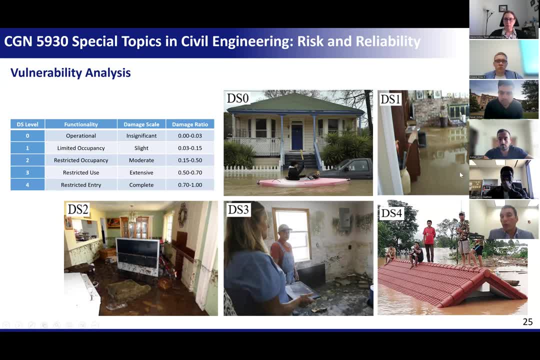 have your carpet width. maybe the flooring is wet as well, so you will have to replace the carpet with some. maybe the baseboard needs to be replaced as well. damage estate two, which include like from one to two feet of flooding inside your home, so maybe your appliances got damaged. your. 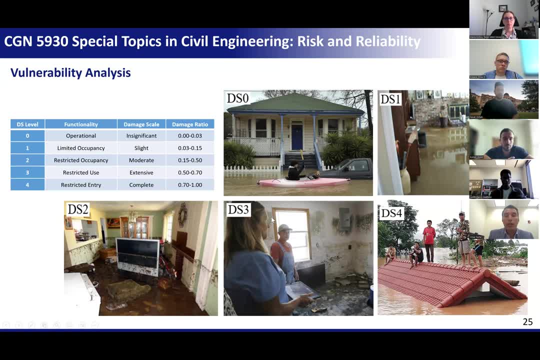 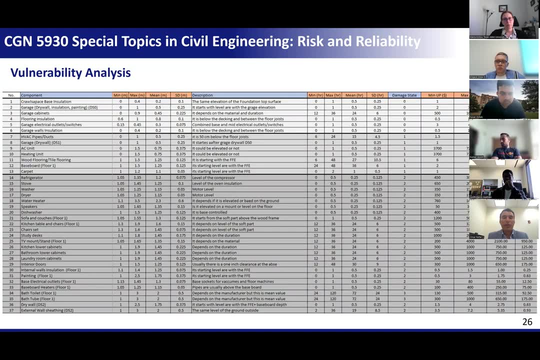 furniture, flooring and drywall, and this is damage estate three. and also we have damage estate four, which is complete damage. this is an example, like from the excel sheet that we developed for the component that shows how we group the component, like from component one to six is damage estate. 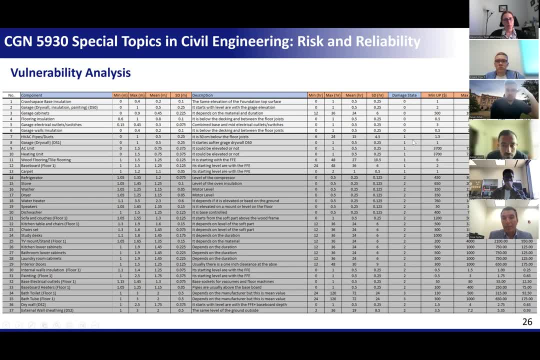 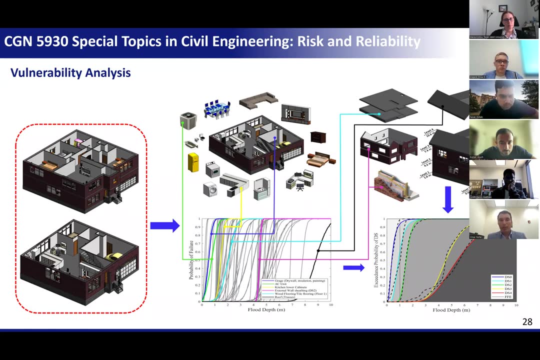 zero here, and from component seven to 13 is damage estate one, 14 to 37 is damage estate two, and we have also three and four and these some of the names of these components. here's it shows how this thing is working. so, as you can see, here we have a one figure that has 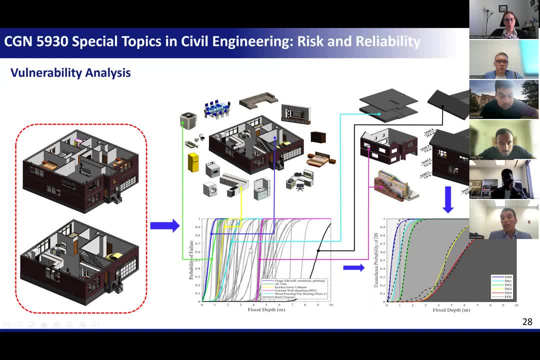 maybe a hundred fragility curve. so this hundred fragility curve is for the hundred components within the building. it tells me what is the probability of failure, for each component was in the building and this was for two-story residential building. and here i like color coded some of these components, so just like. 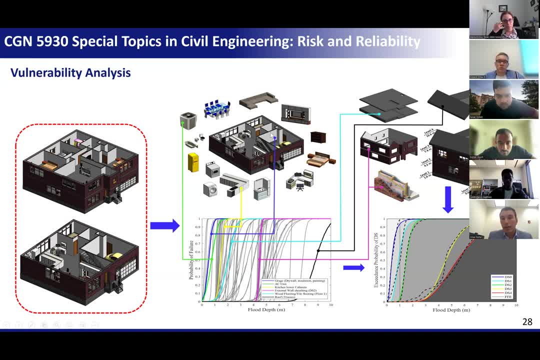 to highlight maybe five of them, including the ac unit, some dry walls, the cabinets, the flooring, and then we were able, through the grouping the the components, based on their contribution to each damage estate, we were able to identify the exceedance probability of failure for each component and then we were able to identify the exceedance probability of each damage estates. it's kind of like 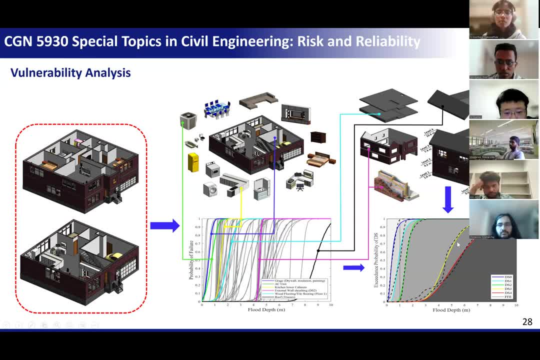 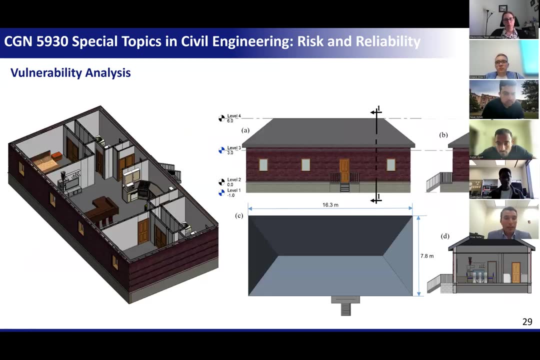 you have a 10 component, contribute, for example, for damage, estate 3. so we make like a weighted average to merge these 10 fragility curves of the com of the 10 components to be a one uh curve like this also. we applied same approach for this is a one-story archetype. here's it shows also. 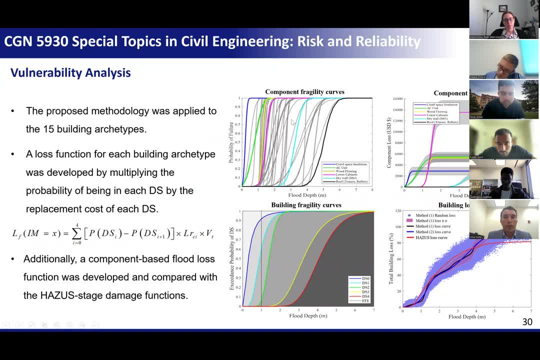 detailed result. um like, here's the component fragility curves. here's some of the loss curves. so basically, if we know what is the failure probability of the component, we can know what is the loss for the component. basically, you multiply the failure probability by the replacement cost of the component. for example, if you have a failure probability of your tv is 50. 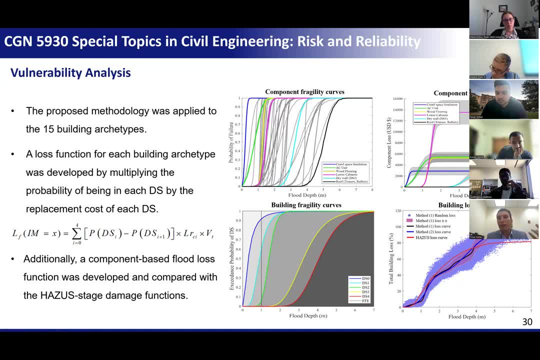 and the price of the tv is a thousand dollar, you multiply 0.5 by a thousand, so the loss will be 500, kind of like probabilistic loss analysis. and here is the building fragility curves which is derived from the loss curves, and the loss curves are the loss curves, which are the loss curves. 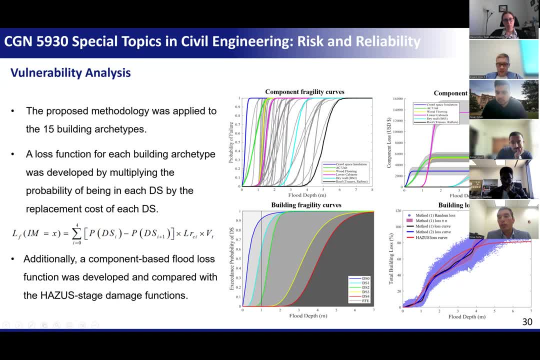 from the components. and also we were able to capture the total loss for the building, like the loss curve for the building at each flood depths. so uh, and also we were able to convert this with what the current standards is using. so most of the the current message is using hazardous stage damage. 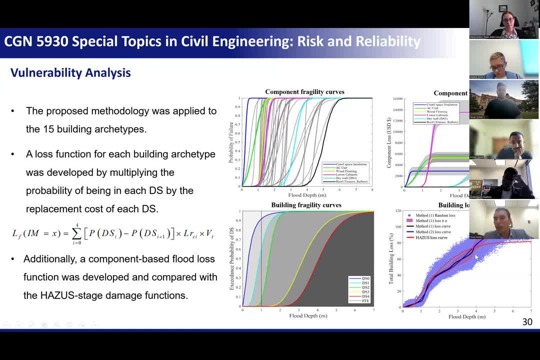 functions and we can burn this with hazards and it shows a great match. at some point there is some mismatching and it has some reasons which explain it very well in some of the publications, because we basically use different approach. hazards, uh, assume that that the building cannot get a hundred. 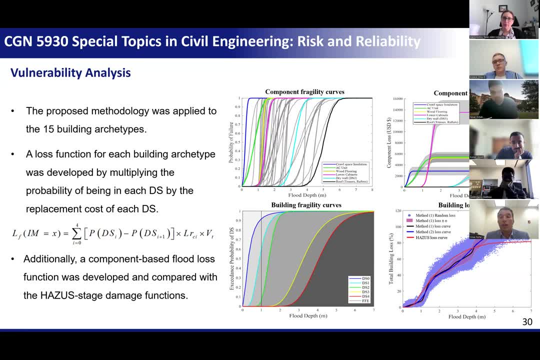 percent damage because you there will be always some components to salvage. but in our method we assume there is a specific uh threshold of water. if if the component reaches so, we consider it as a total loss. so we made the building to reach 100 percent uh losses. uh also, we extended this approach. 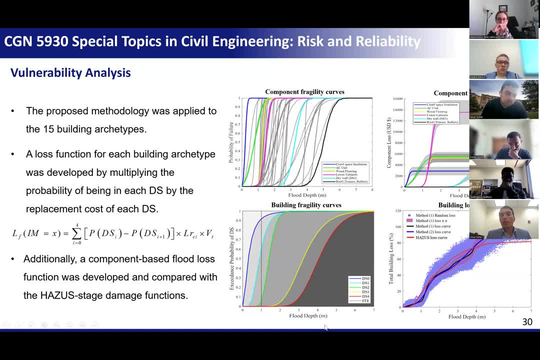 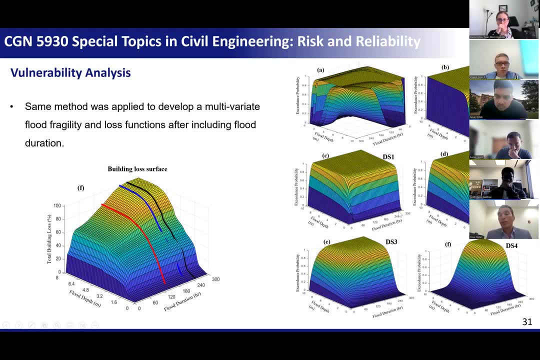 to be multivariate. so, uh, here we only captured the impact of flood depth, so we were able to capture the combined impact of flood depths and flood duration. so right now we are moving from fragility curves to fragility surfaces and from a flood loss curve to flood loss surface. so we did the same thing, but 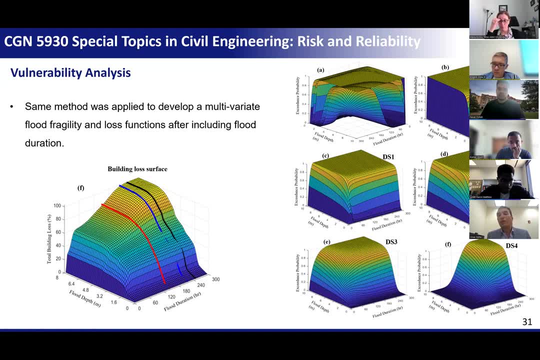 we just like make the flood loss function, uh to be, as a function of flood depths and flood duration, like what is the probability of failure of a specific component if it was exposed for a flood depth of one meter for a duration of 24 hours? so that's um, uh like, um, we're investigated as well. 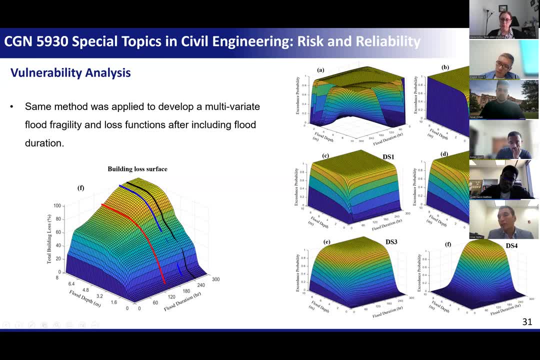 and here's it shows the fragility surface for damage: state zero, one, two, three up to four. and here we have the lost surface for a building. like if a building was hit by a flood: 1.6 meter for the duration of 60 hour- how much loss as a percentage of the total building market value will be. look like: 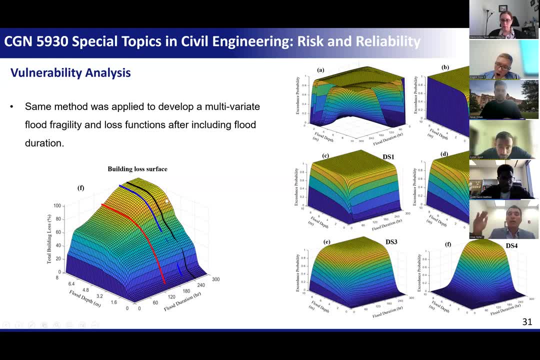 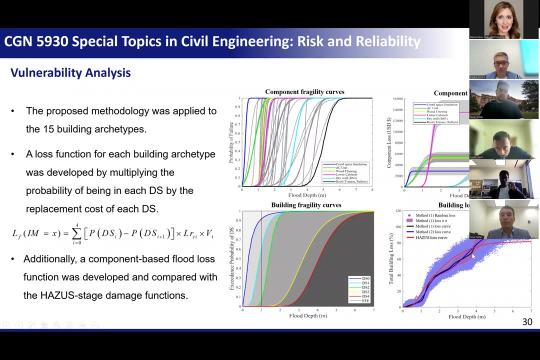 and these three curves are where I plotted the loss curves on the top of the loss uh surface. so basically, when I did the single variable flood loss, I assumed that once the component is reached the um, the, the, the damaging depths, so it will be out of service. so I didn't include the duration. 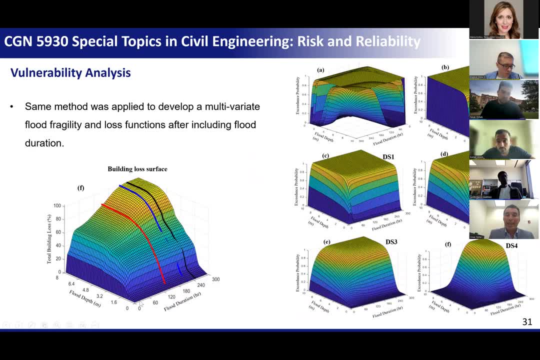 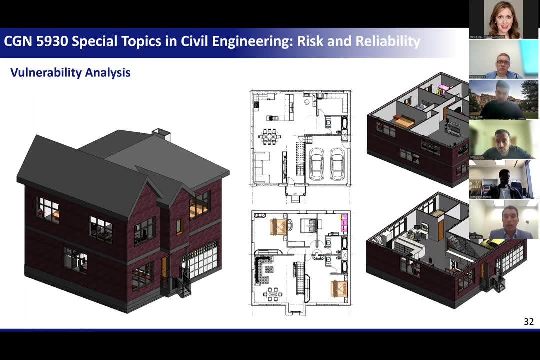 but once I included the duration, so I I can have. if I have less duration, so the losses will be less. but here's my curve. it shows what is the maximum flood loss will be look like. we applied this approach for the 15 building archetype, including. this is a two-story residential building on a crowd with space foundation. this is 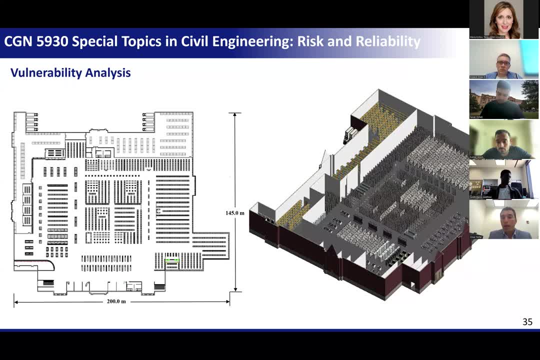 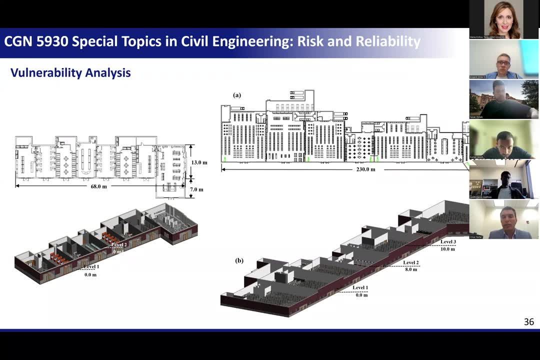 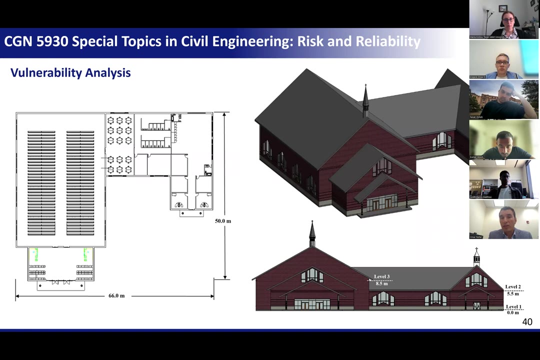 one story residential building, a gas station, a shopping center like Walmart, a strip mall and multi-business buildings and, as you can see, we modeled all the interior content, like if we have like a shopping centers. we modeled the aisles, the fridges and everything uh within uh the building, even office buildings, uh schools, hospitals, uh community centers. 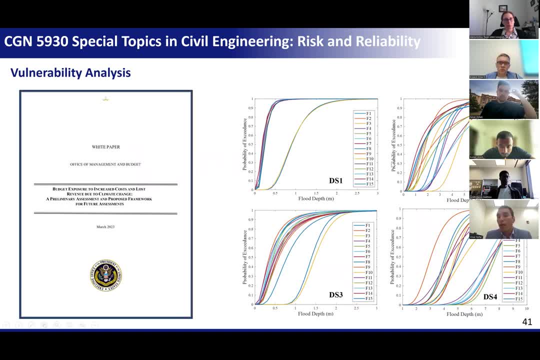 and we have these fragility uh functions. so here's it shows how is the exceedance probability of each damage estate like? we have them just say one, two, three, up to four, and each one of these curve represent a single archetype. this approach has been used by the office of management and budget. 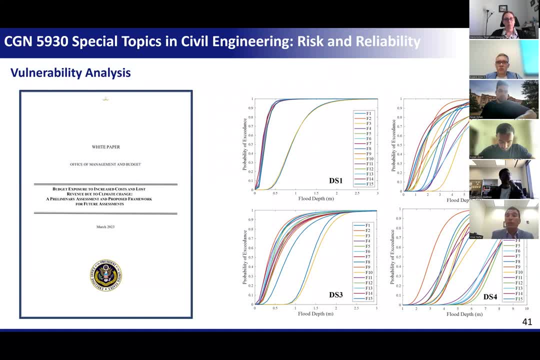 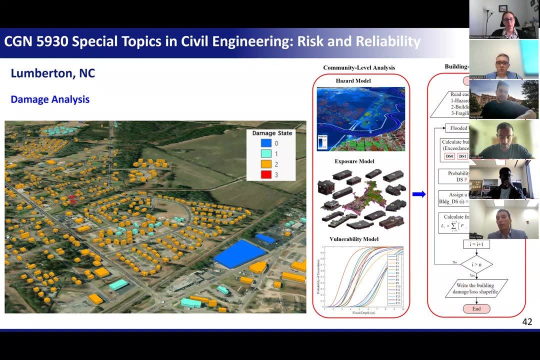 in the White House to um account for the climate risk on the entire US. so this like was impactful to be used by um, uh, the White House, um, so right now, we developed the hazard model and we have an exposure model and we have a vulnerability model and we still didn't do Community level analysis. so what we did, we 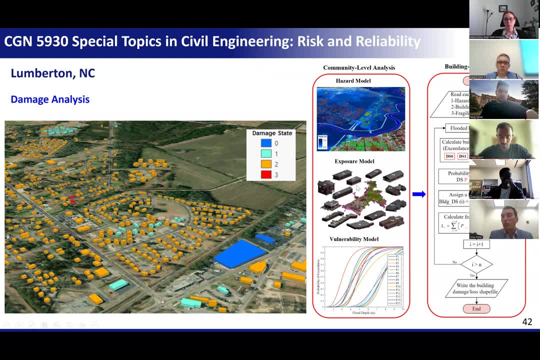 used all these three layers: the hazard maps that we have along with the community, that we developed, and the vulnerability models that we have for each archetype, and then we developed the workload to calculate the hazard intensity at each building and identify what building archetype it is, and then use the fragility function corresponding to this archetype and do building by building. 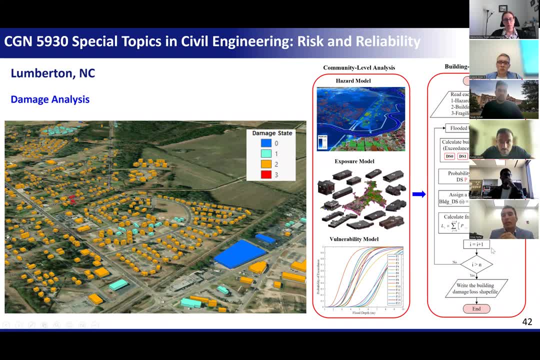 analysis to identify the damage estate for each building. and once we are done, we keep looping one more time to get to the next building until we finish the damage analysis for the entire community. and here's a chosen example. actually, this is uh downtown Lumberton. it shows uh the color-coded map for the building based on their damage estate, like 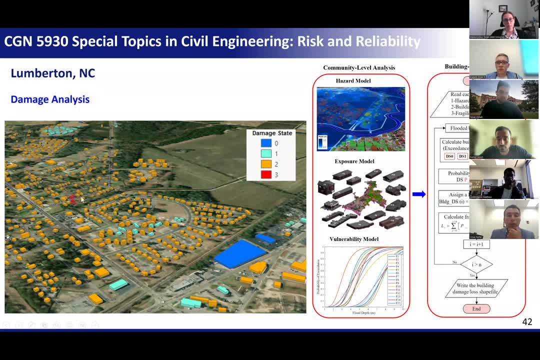 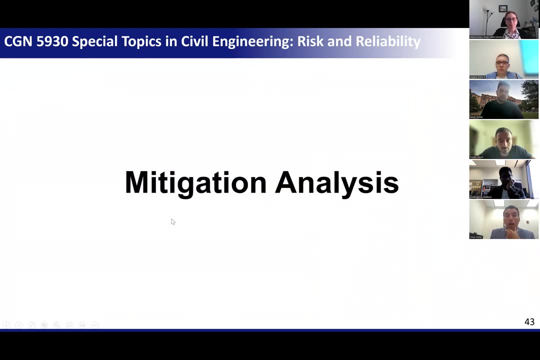 building colored in blue have zero damage, but building in red has like, uh, damage estates three, which extensive damage, but most of the buildings were like in damage estate too, which is like moderate damage. however, there's some as damage estate one as well. with this I'm moving to from 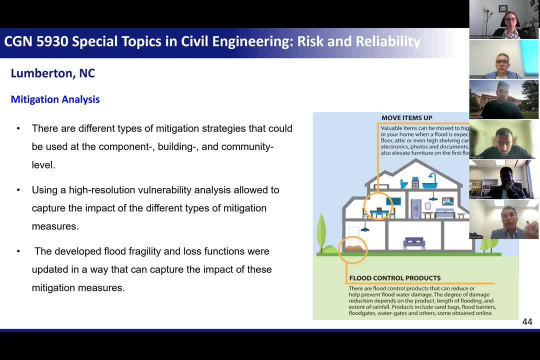 risk analysis to mitigation analysis. so let's see how this approach was impactful when we done mitigation analysis. so, as I said at first, doing uh risk analysis at the at the component level allows us to investigate what, if the household was like, was able to elevate some of the components, like if you have a couch and you put 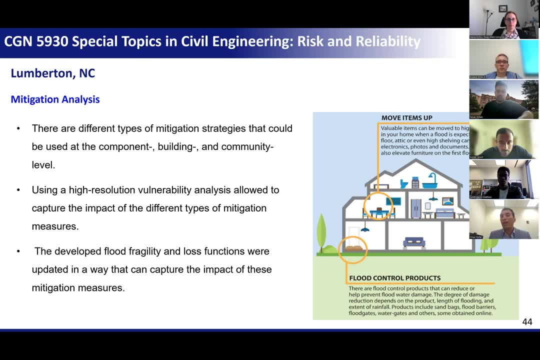 the couch on a higher elevation so that your couch doesn't get wet. if you cleared your entire verse, the story from all the electronics, the gadget, the water sensitive component and you put them in the building, how much loss reduction uh you will have if you were able to um waterproof your building. 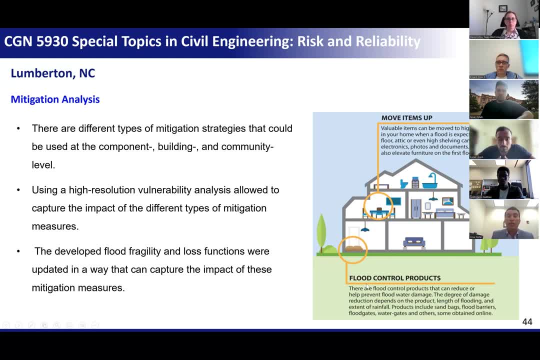 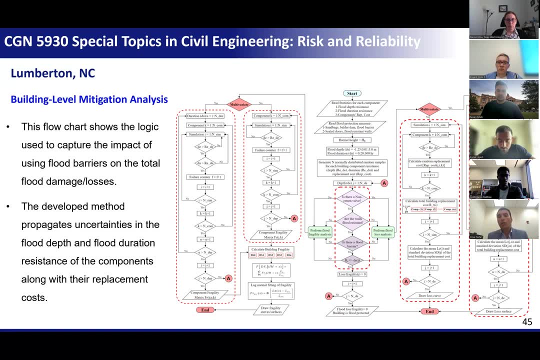 like having a bladder dam or sandbags around your building or even used a water pump, how this is counted. so we developed a very like a long flow chart that shows how all these mitigation measures can be handled. so basically we read all the information about the buildings, about the 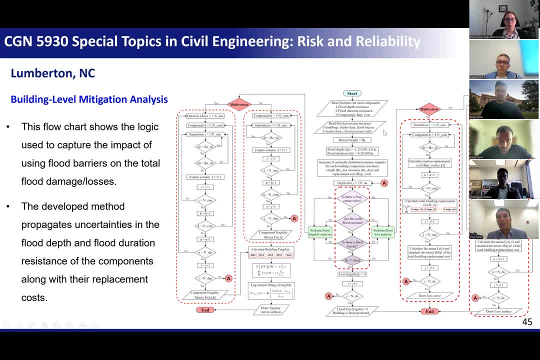 mitigation measures like: if you are using a barrier, what is the barrier height, and if you are using a pump, how long is the pump is going to work. so we've included all of this and identify how much loss reduction that you are going to have with all these mitigation measures. 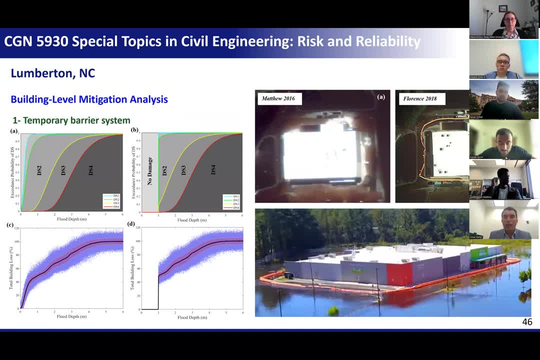 so, um, basically, if you are using a flood barrier, so we model modeled it as simple as that. so, if you have a flood barrier like this, so this is the building without a flood barrier and this is the same building with a flood barrier. so, if the flood, if the water depths is, 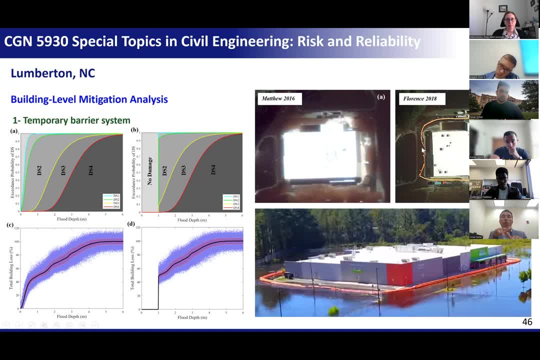 more than the barrier height, so the flood losses will be zero because there is no water will make it to the building. but if the flood depth is more than the barrier height, so the water will overflow the barrier and the barrier will be useless and you will jump back to your original loss function. 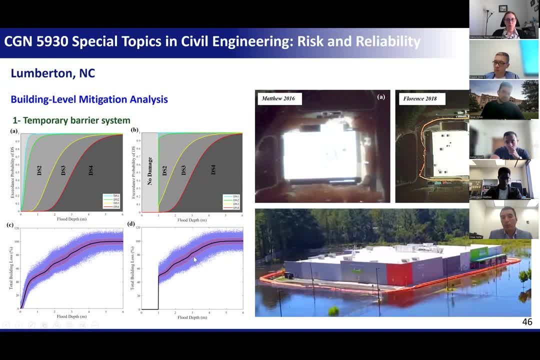 so it's either zero or you will jump back to the original loss curves. so if let's assume that we have a barrier height of one meter, so from zero to one, if, if the flood- this is from zero to one- you exceeds the one meter, you will start jumping back to your original fragility functions. so you will. 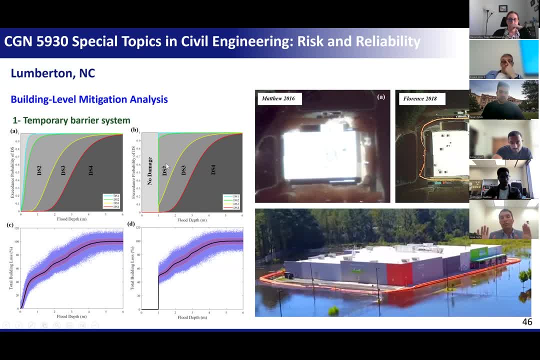 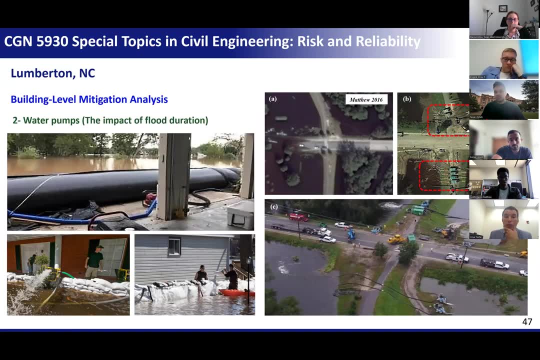 end up with having like damage estate too, because you take the the all the one meter once at a time, because all the barrier is gonna uh fail. uh same thing if you are using uh bumps. we were able also to model using bumps, or using bumps along with barriers, and I'm I'm like showing some pictures. 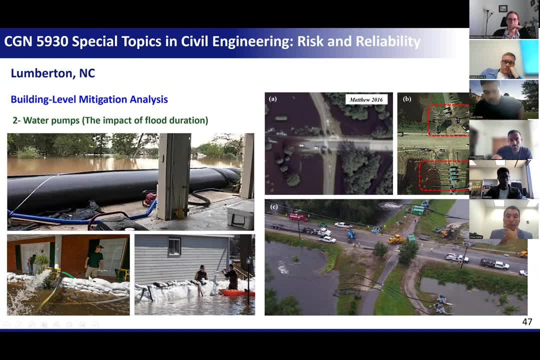 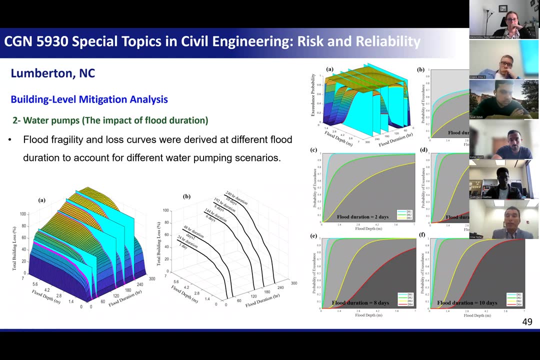 where household were able to have some barriers and have some bumps around to take the water from the property and put it behind, uh, the barrier, so um. so for using water pumps, the 3D function, the 3D loss surface that we developed, has the impact of flood duration. so as soon as you decrease the 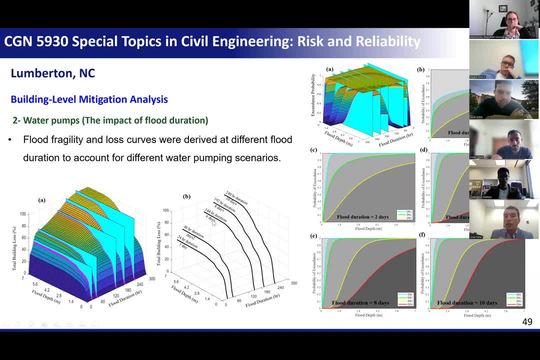 amount of water duration, you are using a completely different loss function. so if your flood uh stays for six days, so the flood loss curve will be this, but if you were able to decrease the flood duration to one day, so you will be able to to use this flood loss surface- sorry, flood loss curve, if you decided to use fragilities also. the 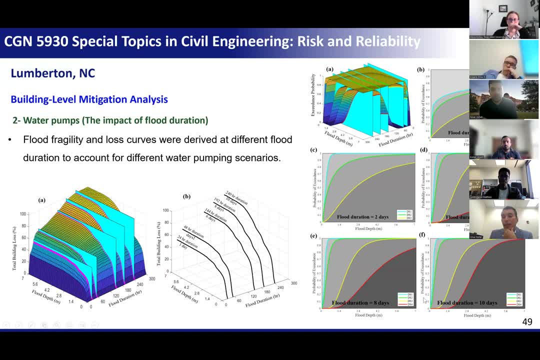 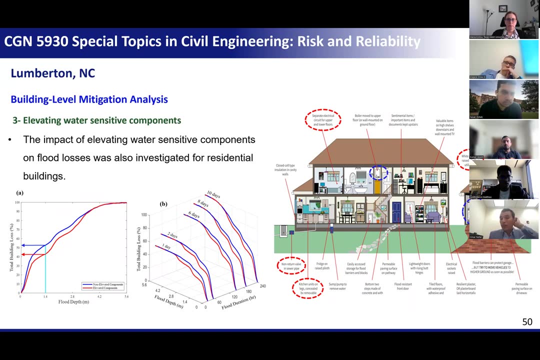 fragility function in one day is different from two days, six days, eight days and ten days. so it's basically: we cut sections in the surface so that we can get these fragility curves. also, we studied the impact of elevating components. so basically, if you elevate the water, sensitive components 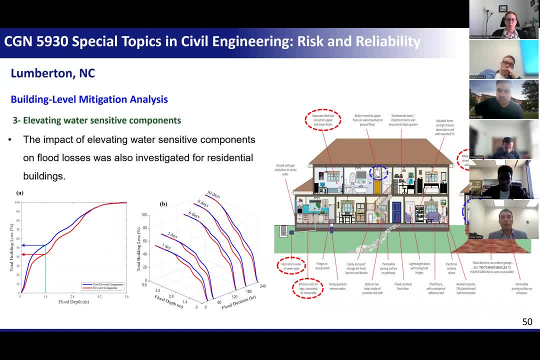 you will not be exposed to flooding at the original uh depths. like the TV, was a diversal floor, so if the water reached maybe one meter, so the TV is gone, but if you elevate it to three meter, to the second floor, so you save the TV. so here's it: shows the blue line, the blue curve, which, without any elevating, 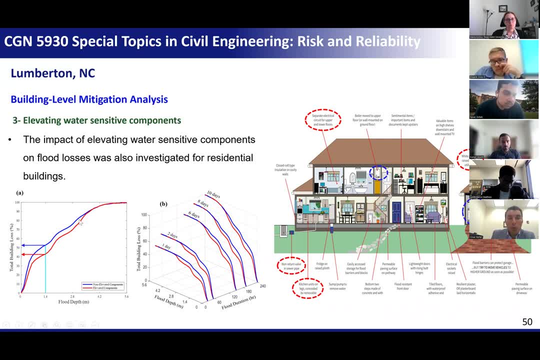 components and the red curve is: if you elevated the water sensitive component, it's not that much, saving the maximum that you can save, but it adds up if you did it at the community level. however, at some point, if you elevate the component, will be useless because if you, for example, 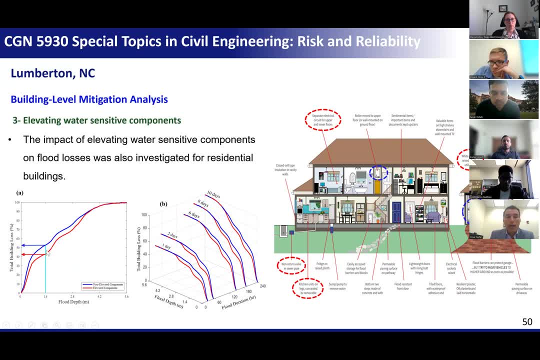 um, having a flood depth of four meter, and what you did is that you elevated, for example, a component that is exposed at one meter flood depths and you put it at the three meter level once the flood hit the four meter. so this component is going to be flooded. so it's, it's um, it's a good. 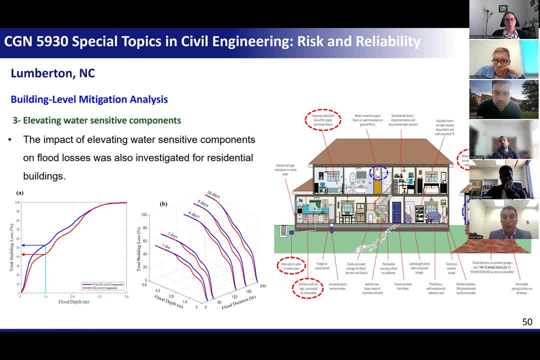 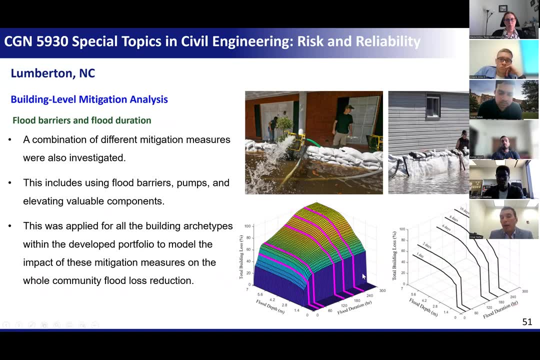 thing at some point, but after that it will be uh, useless, uh, this is like: shows the uh, the combined impact, if you have a barrier and also you are seeing what is the impact, the combined impact, of using a barrier and the pump. so here's it shows. how is the loss curve for each uh one of these? 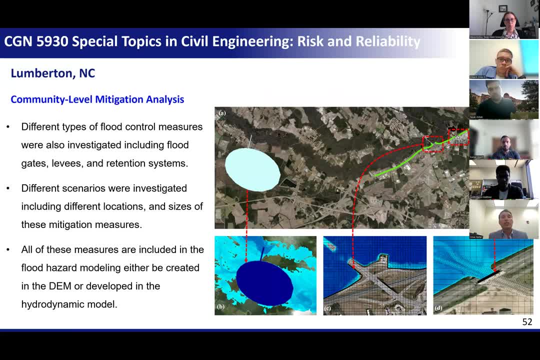 uh. also, we investigated some community level mitigation measures like: what if you were able? for, as I showed at first, uh, this spot allows the water in the community. what if we plug this spot? what we? what if we build a floodgate or a temporary barrier at this location? how this is going to. 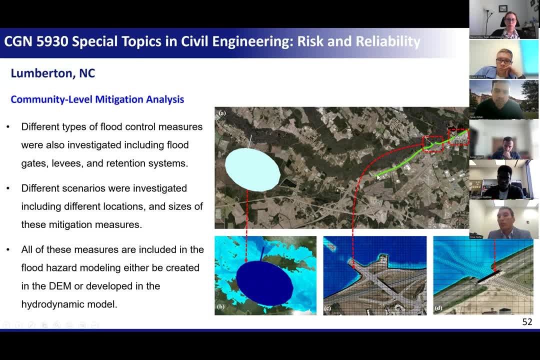 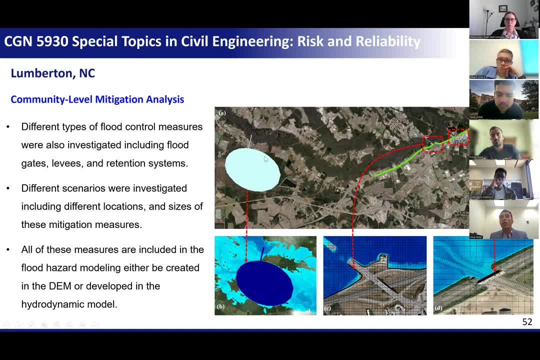 build a retention system. this retention system can take the overflow from the river and store it in in a, in a retention system, and regulate the amount of flow in the river so that we can like when the beak is gone, so we can allow the water to get out of this retention system with uh, with a. 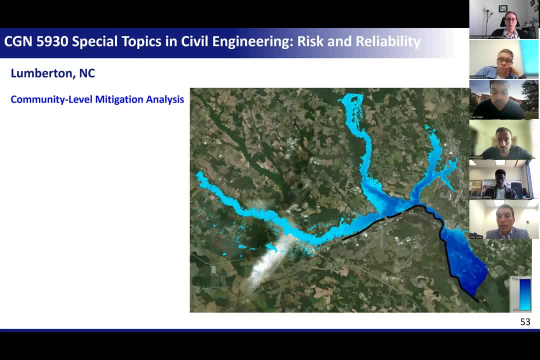 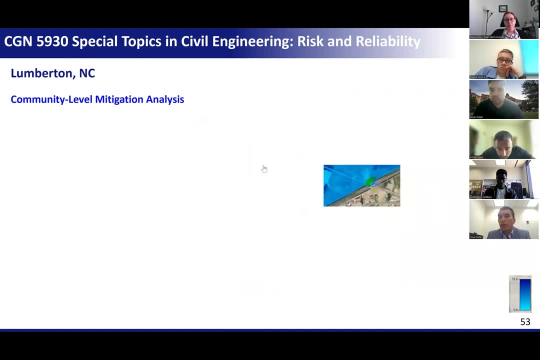 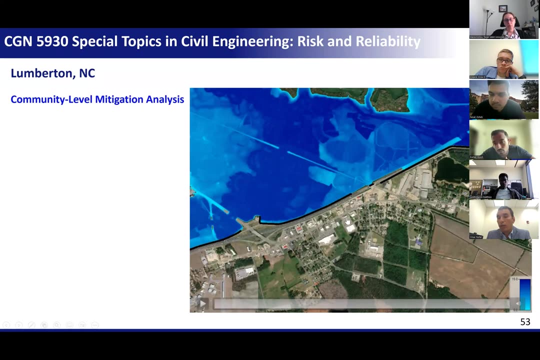 um, we investigated all of this and I'm gonna present uh just one uh scenarios. we we did all uh the scenarios that I I was talking about, so here's it shows uh one of the scenarios: if we built a floodgate and enhancing the levy system, it shows that we provided full protections, uh, for. 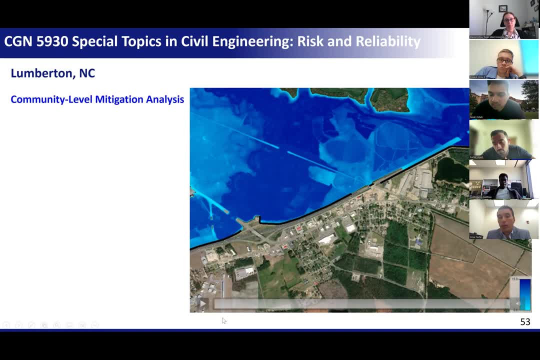 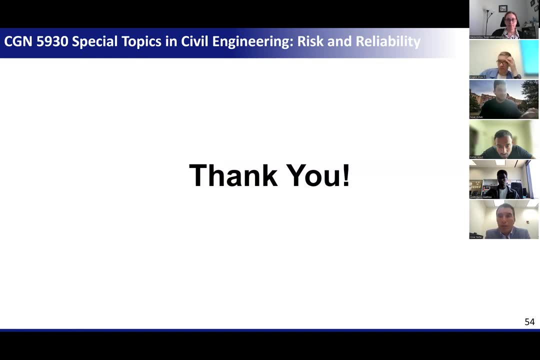 the buildings in the uh floodplain as shown uh here. all right, so with this I'd like to thank you all for listening to my presentation and I hope that you guys like uh understand the concept. I was like a little bit uh fast in some places, but if you have any questions, 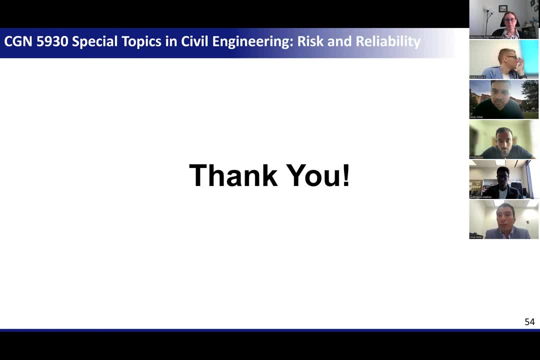 just reach out to me and if you have any questions right now, I'm ready to answer your questions.